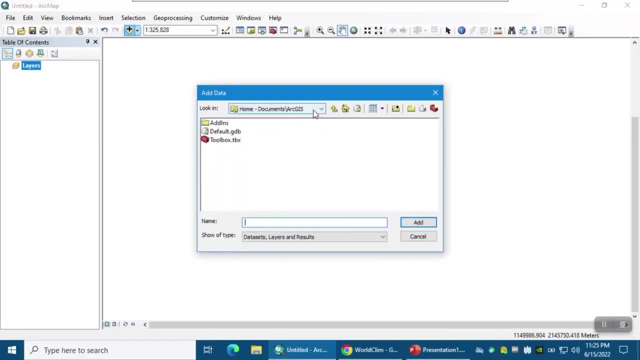 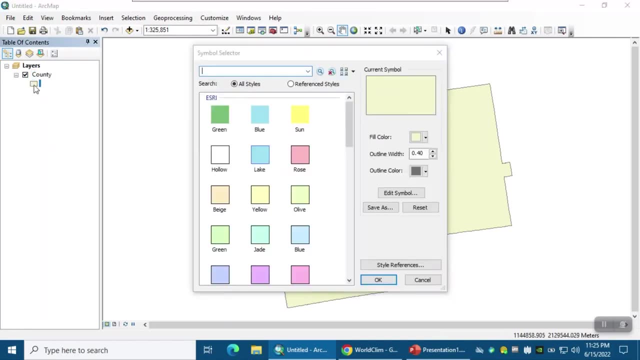 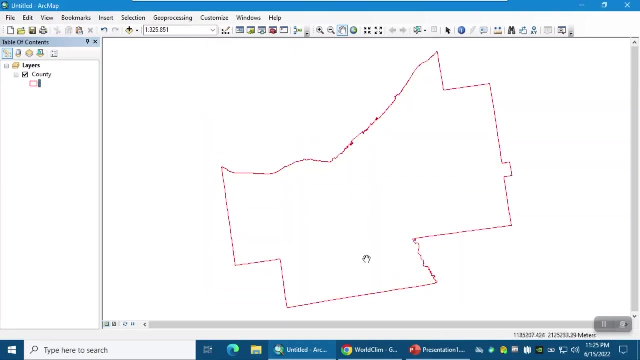 environment. let's add Cuyahoga County GIS flood mapping. Okay, so we have county of the Cuyahoga County. Let me make this hollow, and also I'm going to add the user red color for the boundary of the study area. So that's the Cuyahoga County administrative boundary. 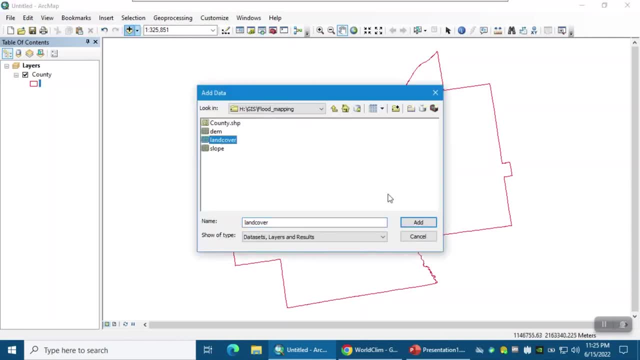 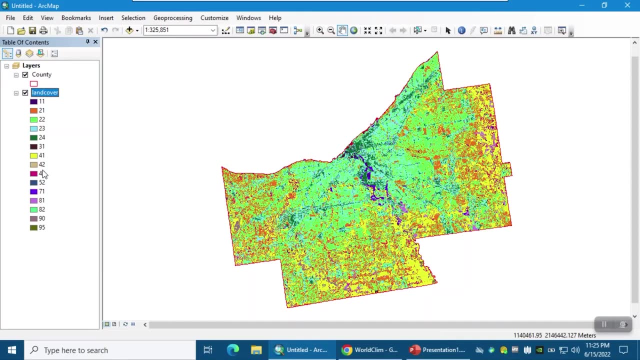 The next one was land cover type. that we talked about that. each, if you load this, each pixel value shows a specific type of land cover. I think the resolution was this: 30 meter spatial resolution. Another factor was a digital elevation model, or DEM. 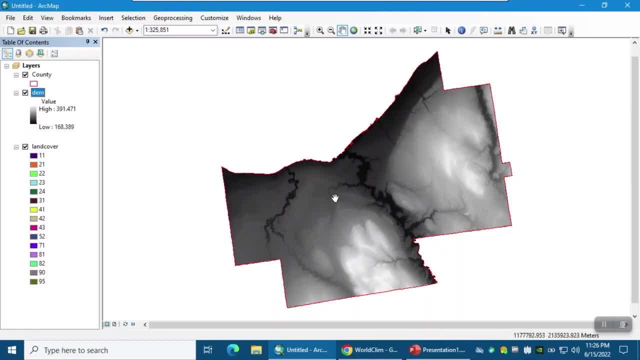 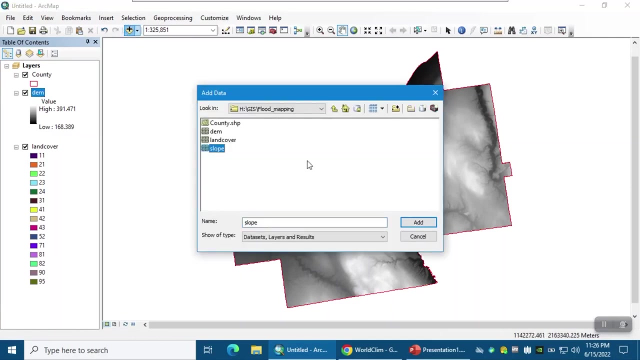 When you add that each pixel shows elevation for that specific location and again, the spatial resolution was 30 meter and the elevation varies from 168 meters to 391 meters in the city area. And also we derived slope from the digital elevation model and, as you can see, the slope changes into the area, So it's very difficult to see where the elevation is. So this is an easy way for us to see where the elevation is. So that's it. Thank you very much. 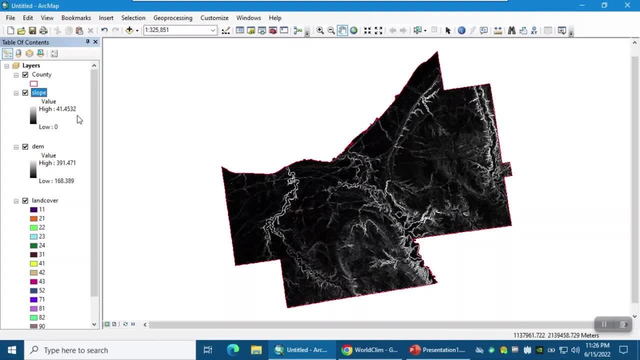 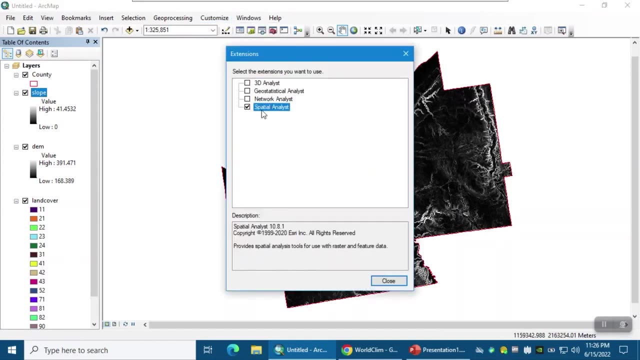 changes from 0 to 41 degree, that we already talked about that in the previous slide, that how we can drive the slope from the digital elevation model. the next factor is precipitation. but first let's from customize menu go to the extension and then check a spatial analyst on. 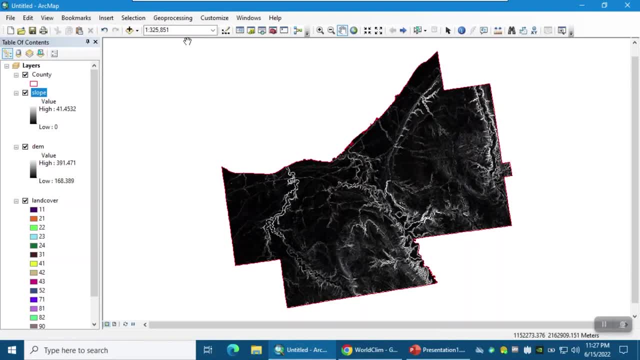 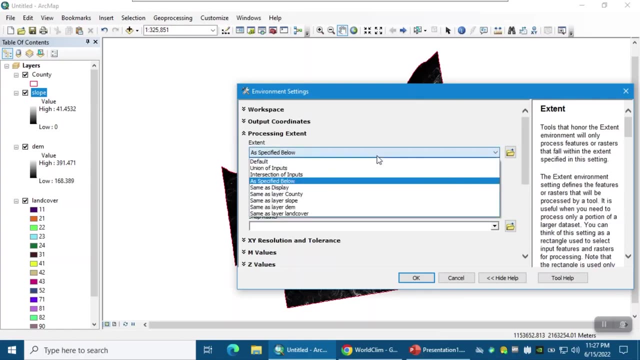 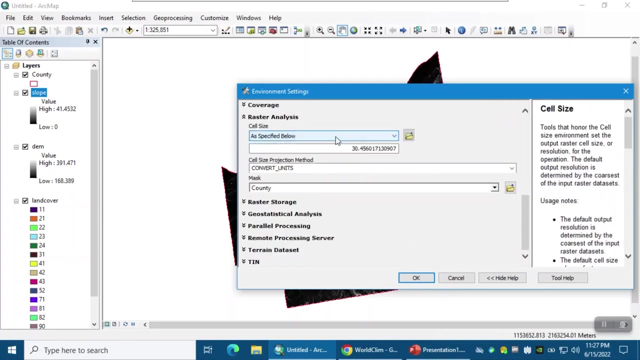 and after that. and also you have to limit the process. we want to limit all of the calculations to this study area, so from geoprocessing and then environments. so if you go to the processing extent, we're gonna set the extent as same as county layer and also the cell size as digital elevation model. 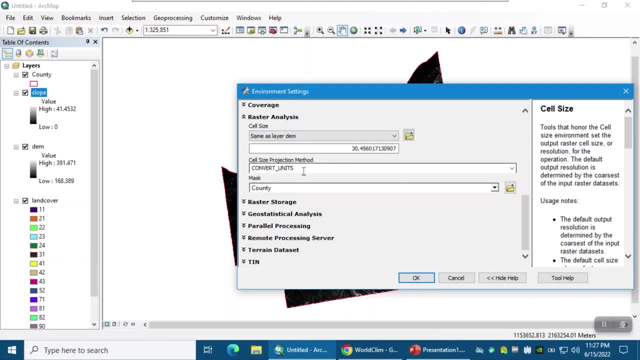 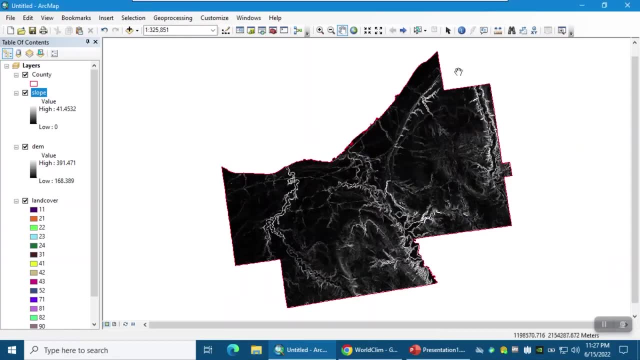 so same as slope or digital elevation model, and also we want to use the county as the mask. okay, so click. ok, so we don't want to do any calculation outside of the study area. okay, so, regarding precipitation, we can get the precipitation information from worldclime website, if you. 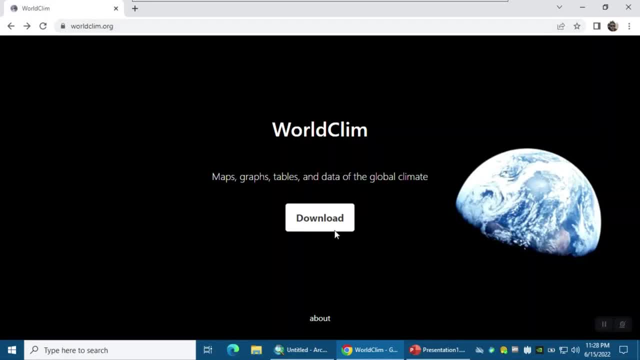 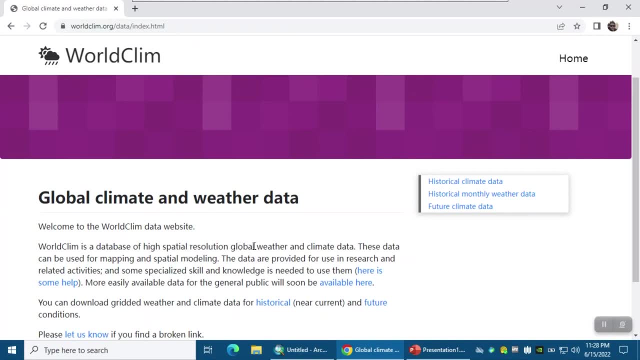 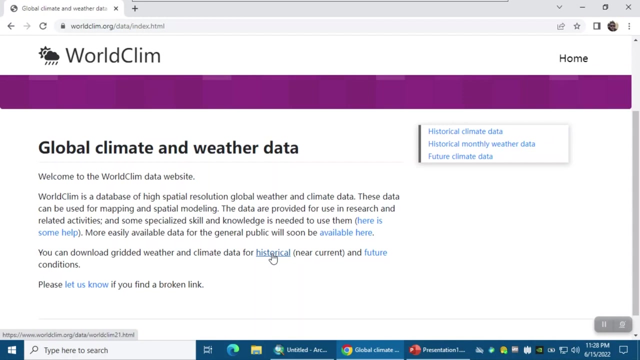 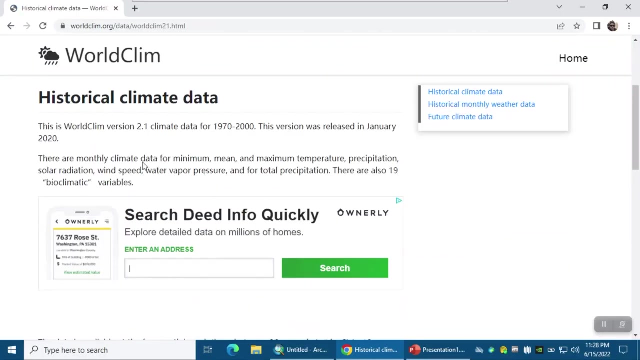 go to the worldclimeorg and then click on download. so worldclime provides relatively high spatial resolution global weather and climate data. okay, and it is highly. it is extensively used in spatial modeling so we can get the historical information of the climate or weather condition. so if you click on historical and after that this website provides the monthly climate. 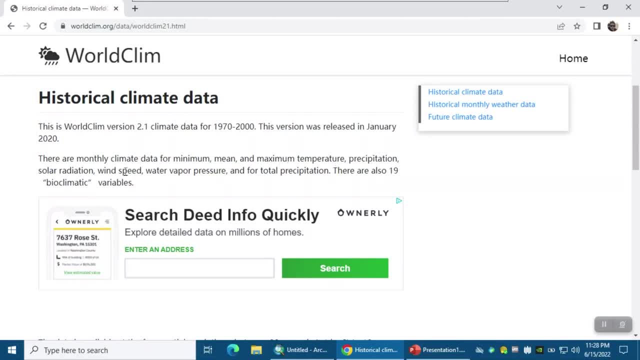 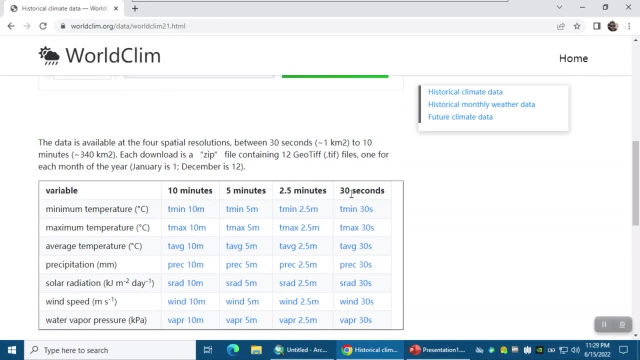 data for minimum, mean, maximum temperature, precipitation, solar radiation and so on. okay, so here we have the variables and also here we have the resolution. so the best resolution is the resolution, which is the one square kilometer. so i'm gonna download the precipitation: uh, with 30. 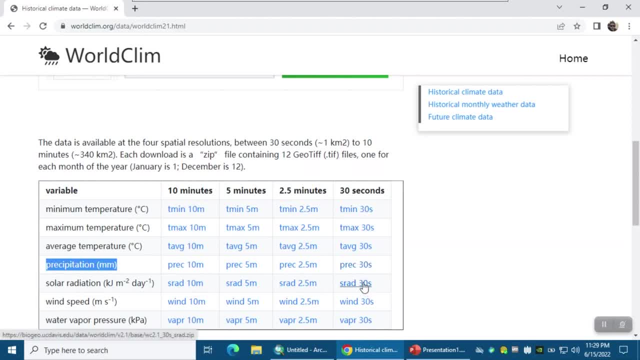 second or one kilometer spatial resolution, which uh provides the data and, as you can see it's, the values are between 1 to 12, so it's a monthly information, so let me click on this one and download it. so there's gonna be 12 raster grid and we're going to focus on march. 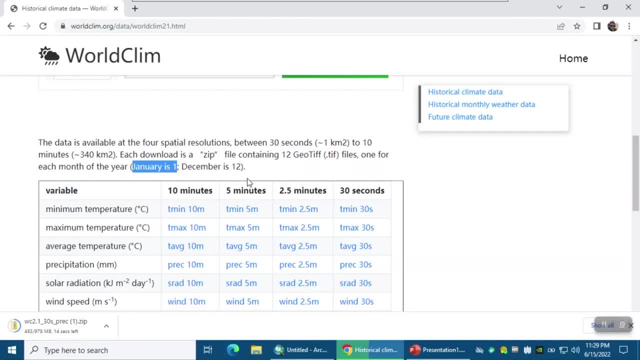 because, uh, most of the floods occur normally occur during march, and because of the after snow melts and because of the rainfall. so i'm going to focus on only for the march months and consider it as the precipitation. so, if you uh open up this file, so i already have. 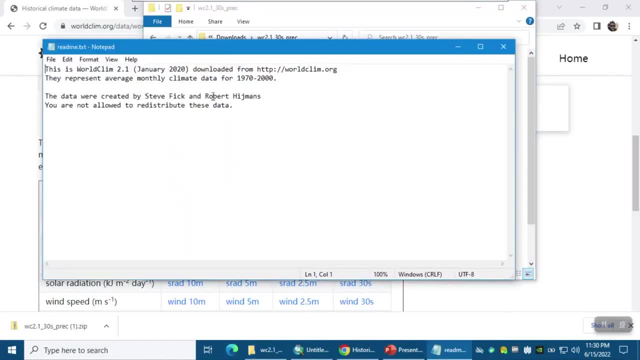 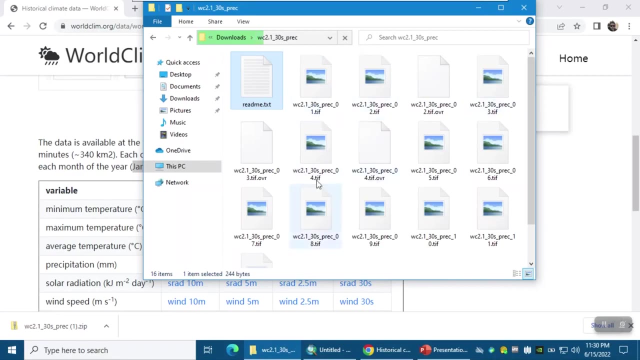 unzipped this file so you'll notice that if you click on with me. so it shows that they represent average monthly climate data from this period of time. okay, so, uh, we have the value from months one, two, three, uh, four and so on, so we're going to focus on month three, which is march, and the data. 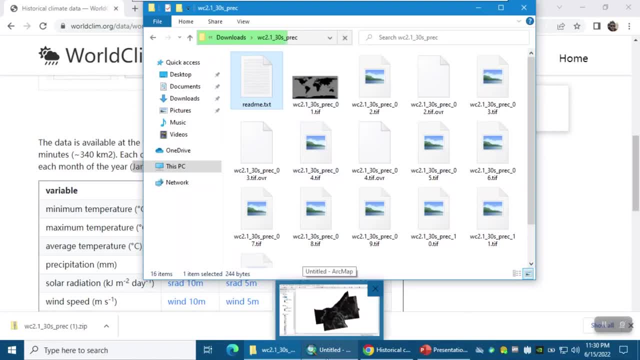 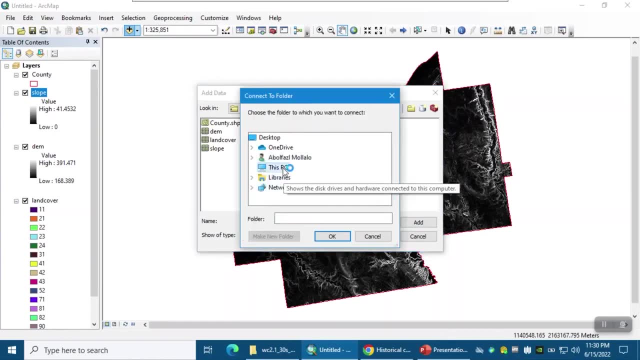 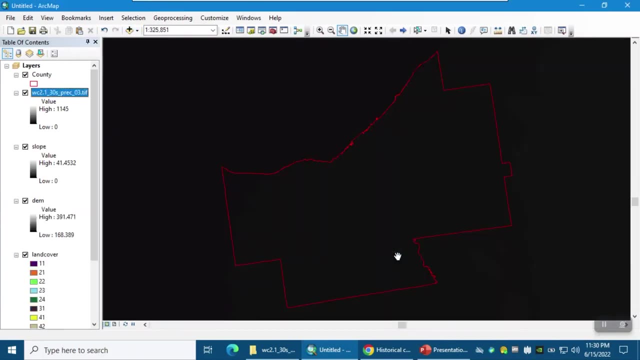 are for the entire word. okay, so we have to clip it with our study area. so let me click on add data and then connect to folder of the downloads. I'm gonna select the month three and then add so you can see it's for the entire word. if you click on full extent is for the entire word, but I'm gonna 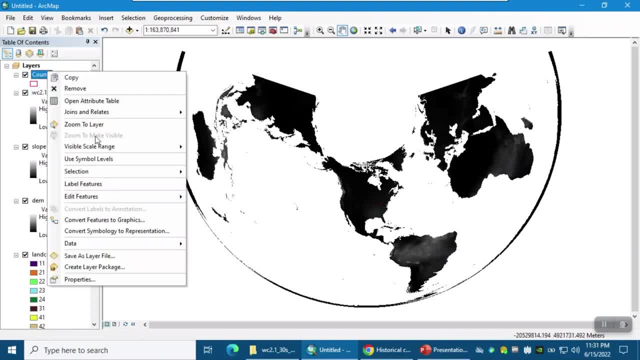 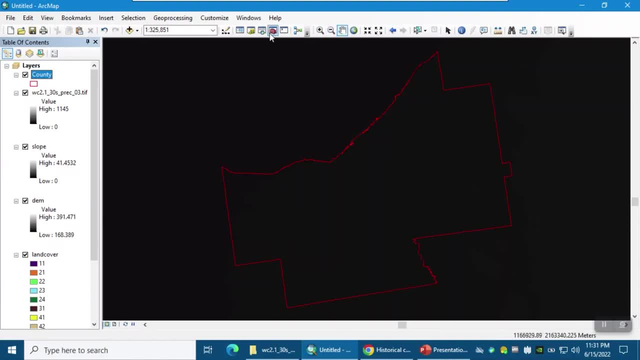 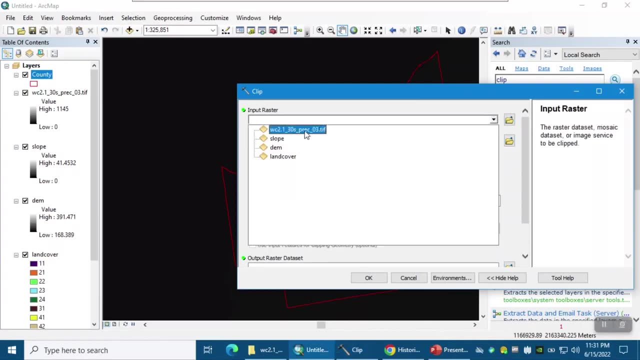 just focus on Cuyahoga County. so let me zoom to this layer. I have to clip this big raster with the Cuyahoga County, okay, so if I type clip here, clip data management, so input raster is gonna be your precipitation for March and the. 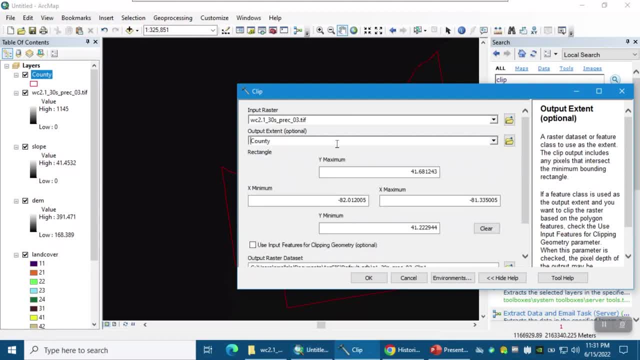 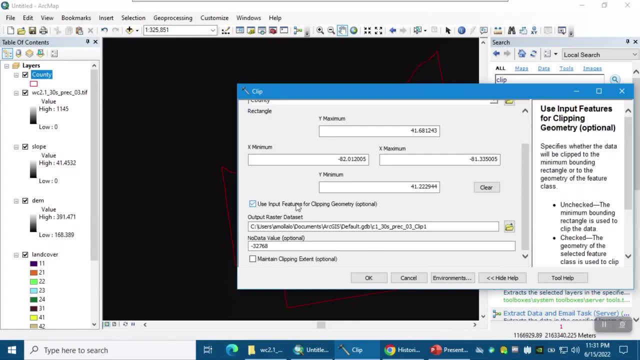 output extent is gonna be for County and after that we have to. we want to use input feature for clipping geometry. okay, so if it's checked, the geometry of the selected feature is used to clip. so it's gonna be for the Cuyahoga County. so we. 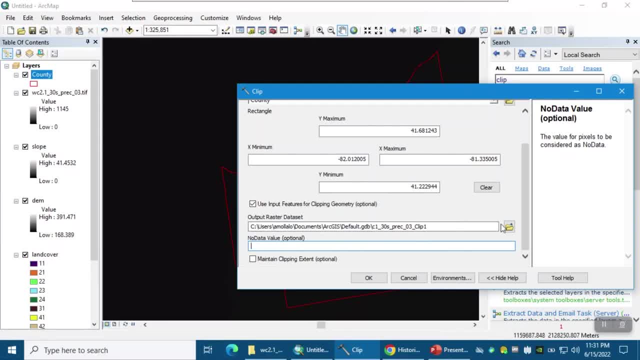 don't need to convert this to no data to this value and I'm gonna save this as PRC precipitation and I'm gonna save this as PRC precipitation and I'm gonna save this as PRC precipitation. so that's the precipitation for Cuyahoga County, and maintain clip extent. 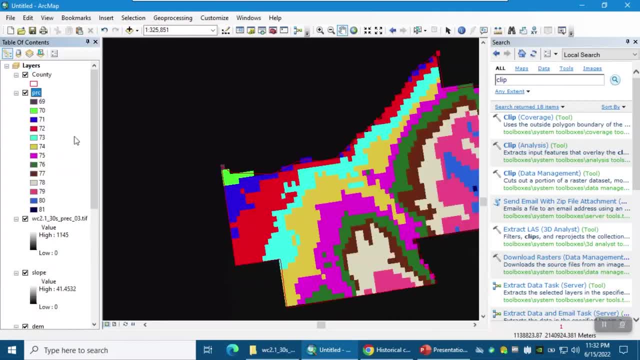 and then click OK. so, as you can see, here we have the precipitation, but the resolution is not perfect. that's one of the limitation of this data: that when you have the data for the entire word, the spatial resolution is one kilometer, is not 30 meter like the other variables that we have, but the 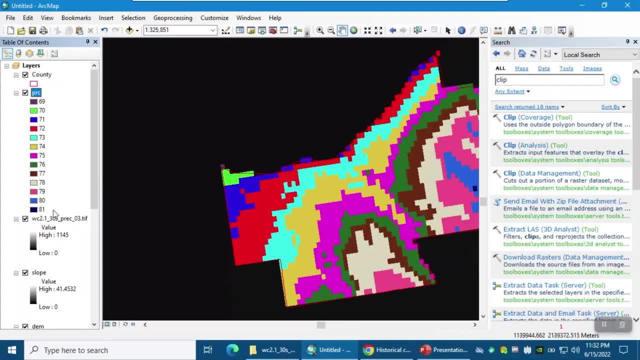 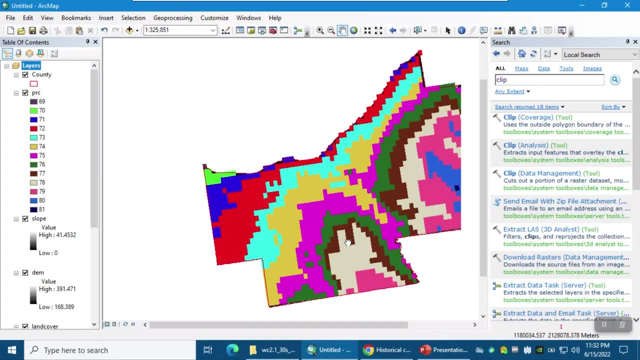 so that's going to be our precipitation layer, so I'm gonna remove this one and only consider this as precipitation. so, before extracting, before focusing on the next variable, which was proximity to streams or channels, let's look at the hill shade of the study area. so what is hill shades? let me 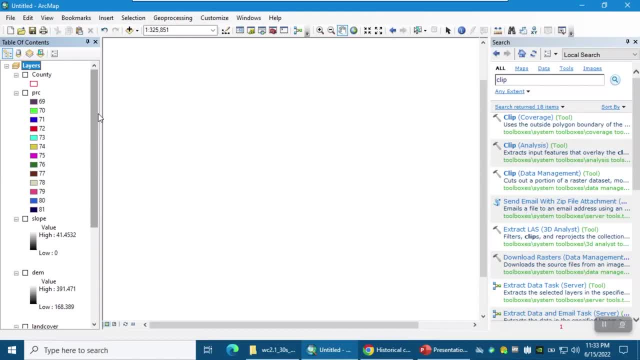 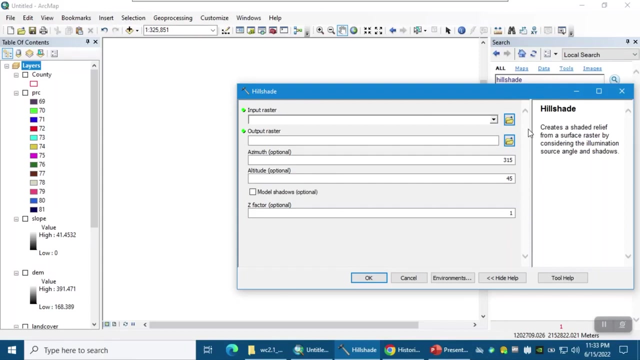 turn all layer off. the hill shade provides a more clear picture of the topography. yeah, because it mimics the sun effects on hills and canyons. okay, so if you here, if you type hill shade and hill shade, spatial analyst, so your raster input is going to be your digital elevation model. 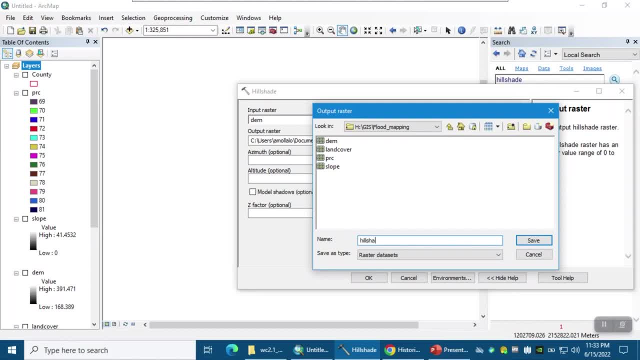 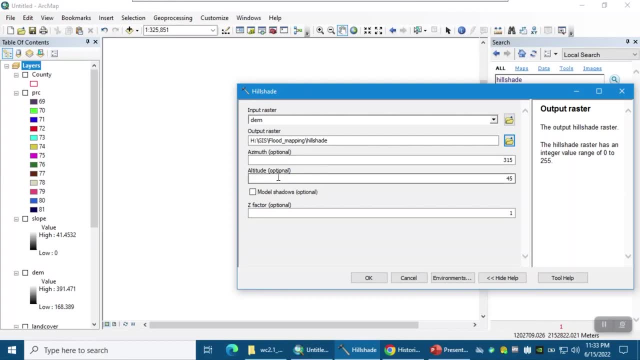 the output is going to be your hill shade, and so these are these two. azimuth and altitude are for lightning sources and optional information, so i'm going to accept the default values for the hill shade and after that i'm going to click okay, all right. so now here is. 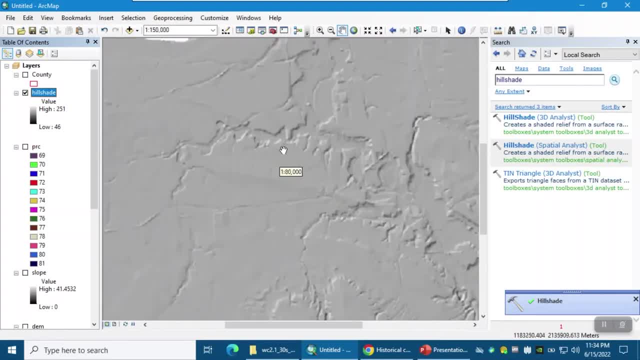 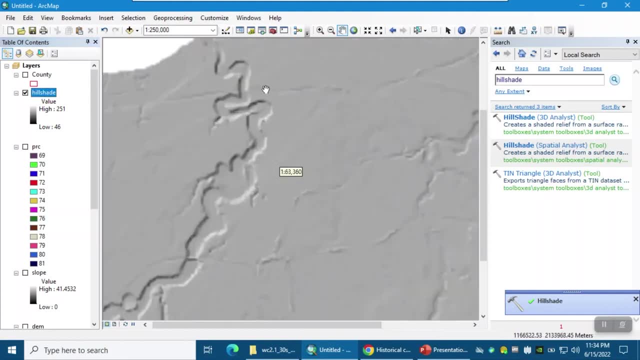 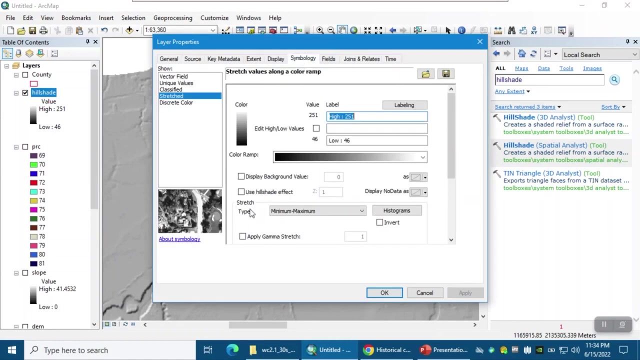 hill shade. if you zoom in you can see the details of landscape, so it's like almost 3d image. okay, so here you can see the known variations of the landscape, but if you want to see better, better the variations in the hill shade, if you right click on hill shade properties, go to the symbology tab and 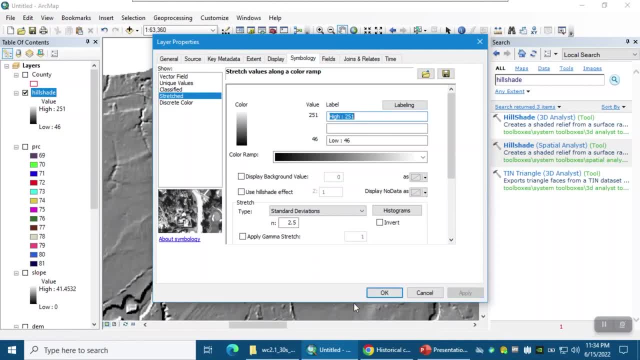 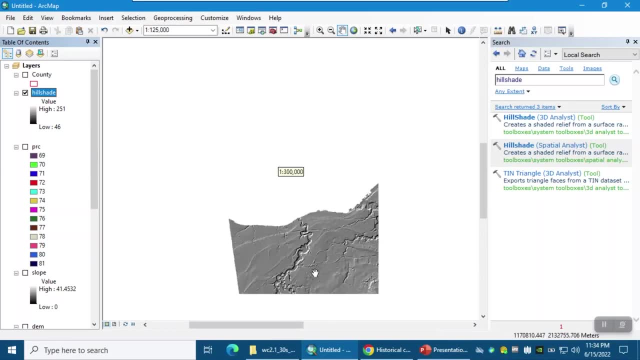 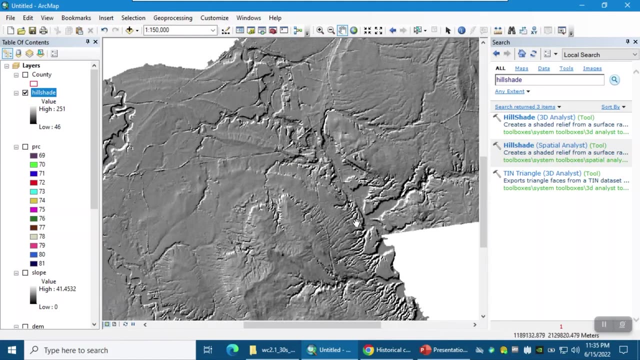 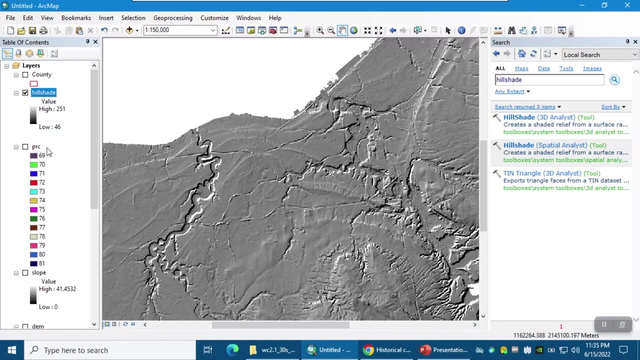 stretch it based on standard deviation and then apply: okay, you can have a more clear picture of the topography, okay. so here probably we have some depression, we have some channels so you can better see the uh, the topography changes of this study area. so let me add the land cover uh to on top. 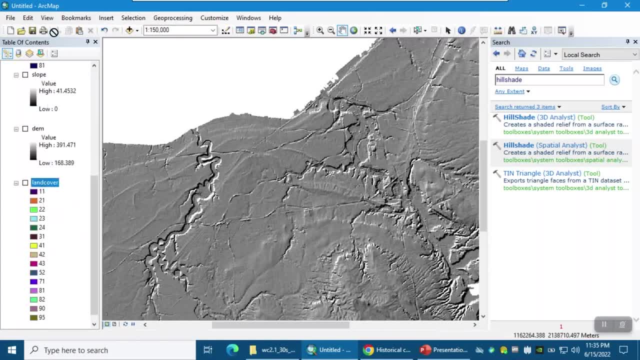 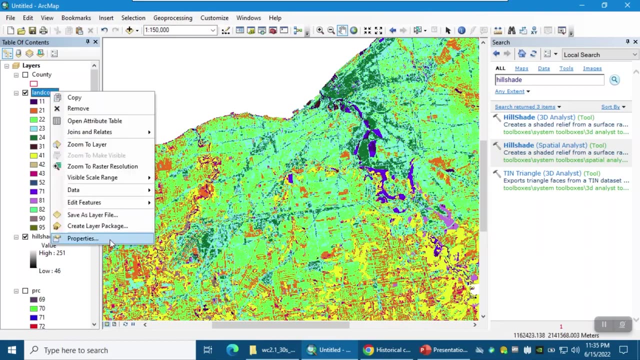 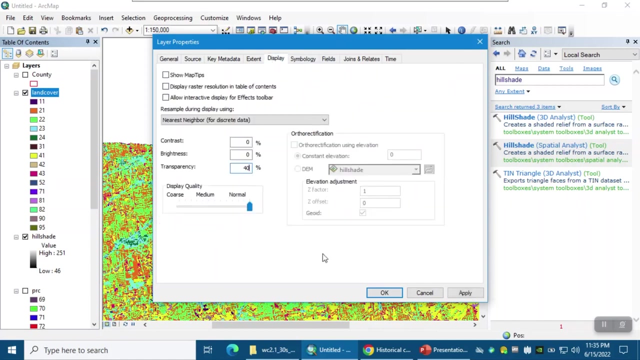 of this layer. so we had land cover here. i'm gonna move it on top of the hill shade here and then, uh, what i'm gonna do is i'm going to, in increase the transparency of the land cover. okay, so right click on that properties to display, and then, for transparency, i'm gonna increase it to 40 percent and then apply and okay, 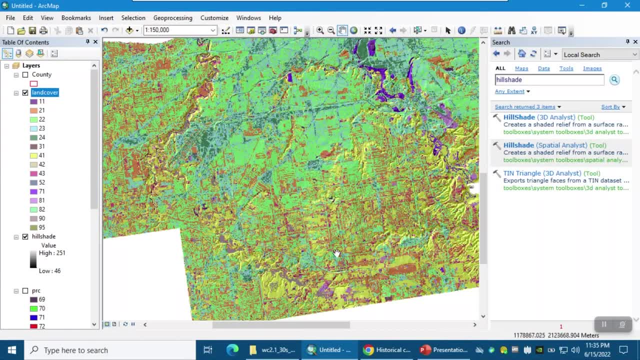 so here we can, so you can see land cover, 3d land cover map, kinda. so this map is called shaded relief map- is a 3d, almost 3d, form of the land land cover. so this is how the landscape look like. so we don't need this hill shade, uh for our analysis, but we just wanted to have a representation. 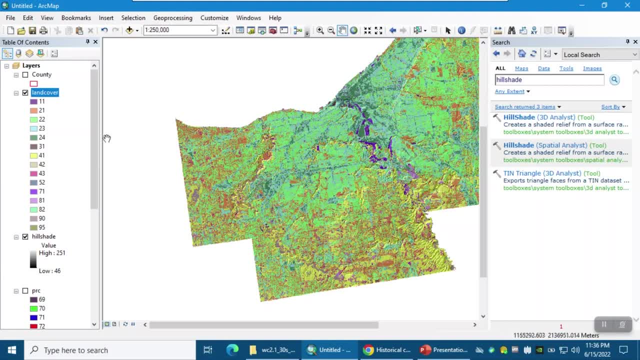 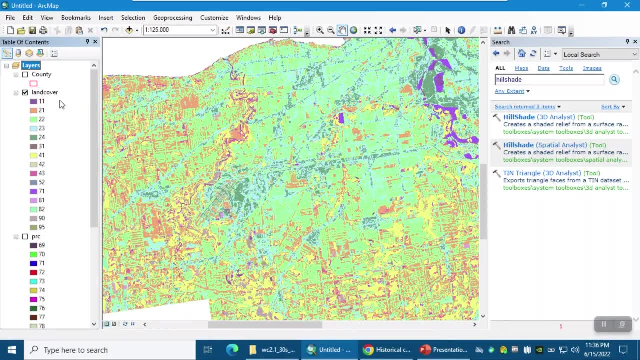 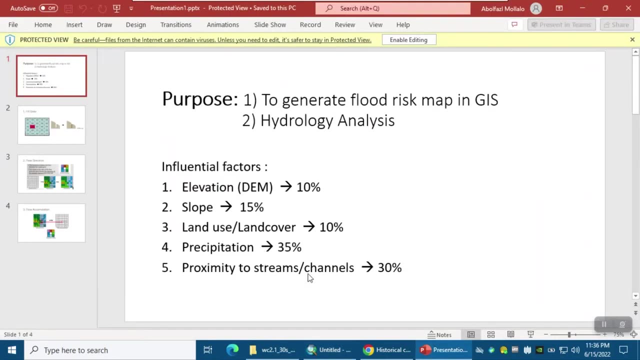 of the land, uh, landscape, so we can remove it for from our analysis. so let me remove the? uh hillshade, uh, okay, so, uh, the next step. so we have the elevation slope, land use precipitation. the last one is proximity to streams- right, so, uh, we want to extract streams from digital elevation. 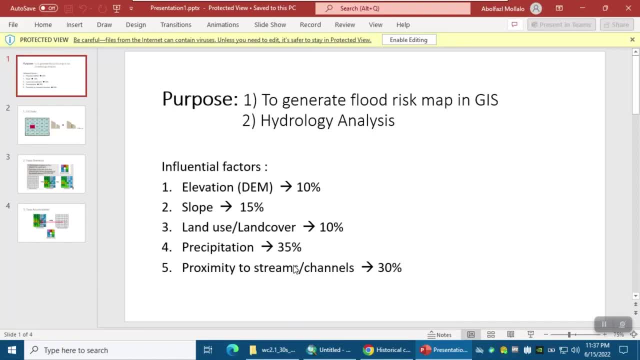 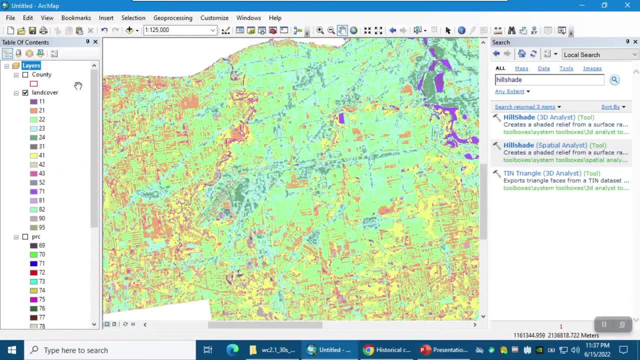 model, but there are multiple steps that we need to take, uh, to extract streams from digital elevation model, but there are multiple steps that we need to take to extract the streams or channels from digital elevation model. okay, so let me remove all layers. we can add them later. so let me select all layers and then 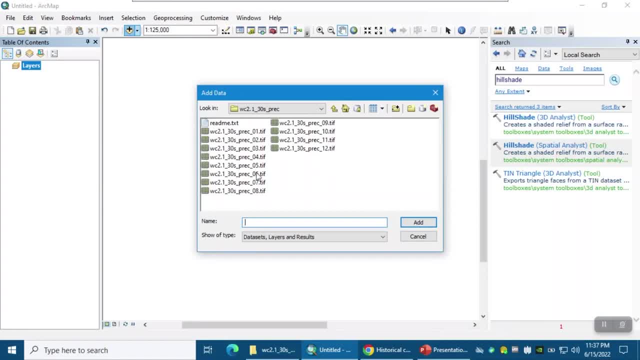 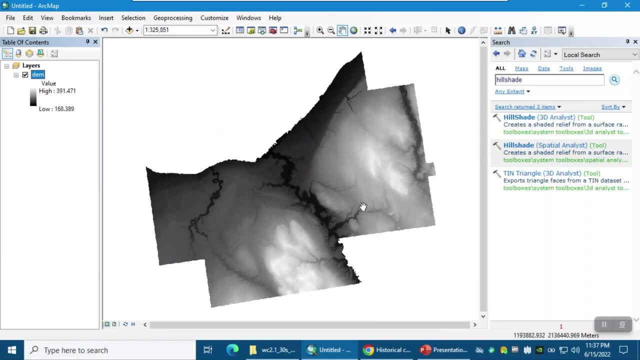 remove it. okay, so i'm gonna just keep the digital elevation model, okay. so, uh, in your digital elevation model, uh, the first step is that we have to fill the digital elevation model. and what does it mean? so in your digital elevation model, there might be some sinks or pits that are pixels that are lower. 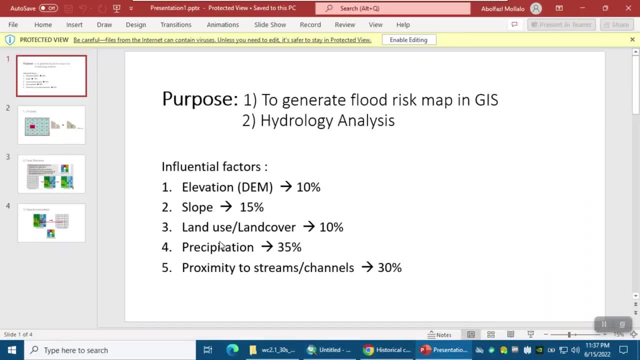 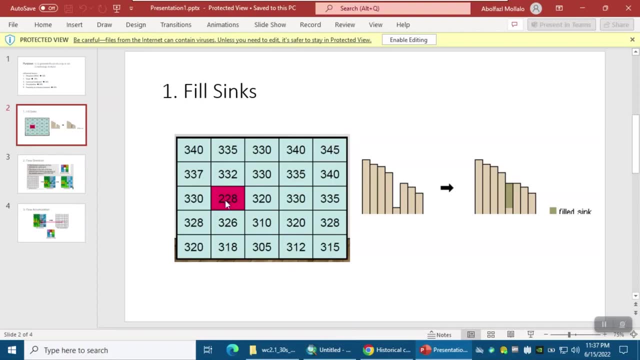 than surrounding cells. okay, so here, if you look at this one, so if you look at it, so if this is the elevation model and each cell represent elevation, so some pixels are significantly lower than surrounding cells. okay, so the problem of sink is water will trap in these cells. okay, 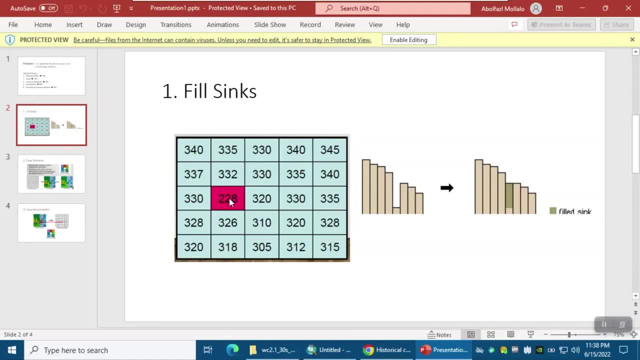 and these spurious things are found in most digital elevation model products because of the small, random errors in data collection and the field function, as we can see, helps us to modify the elevation value to eliminate these problems by filling the artificial sinks in the digital elevation model. okay, so we need to fill the digital elevation model. 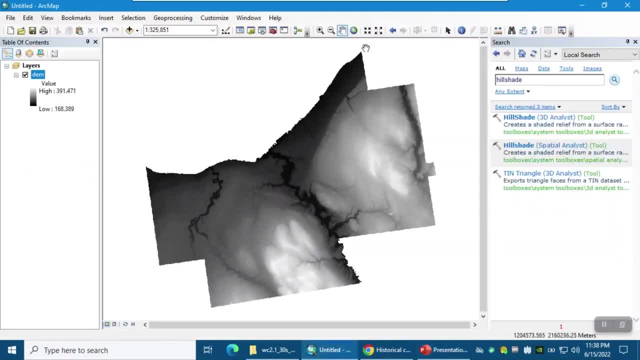 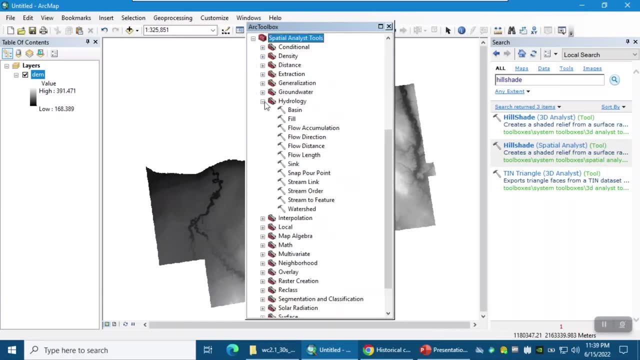 and do that if you go to the arc toolbox here and then from our toolbox, if you scroll down and find spatial analyst and then the hydrology extension, expand the hydrology and then here we're going to focus on this hydrology extension. okay, so the first operation is fill and the fill the input. 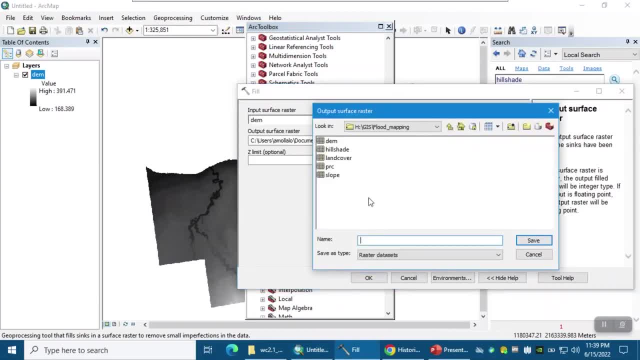 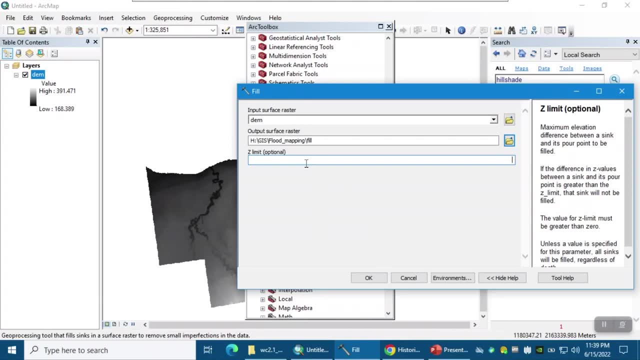 is going to be your digital elevation model and the output is going to be fill. okay, i'm just going to call this fill and z limit. what is that limit? because, uh, in order to differentiate natural and artificial sync. okay, sometimes you have natural, you have something, but sometimes you have. 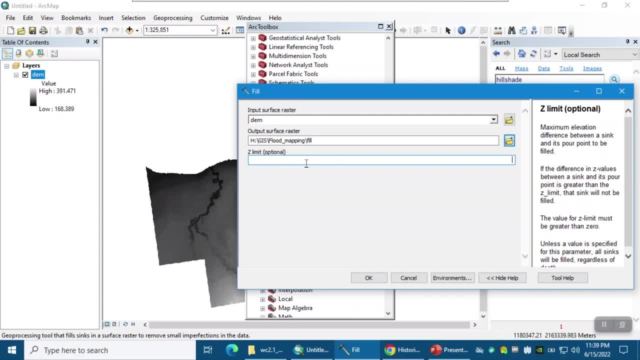 uh, things because of the errors. it's an artificial thing, so we need to set up a threshold value for errors under. for example, if i put the value of 10, the values that are under 10 is going to be filled, you okay, and above, that is considered a natural sync and should not be filled. and here also explains: 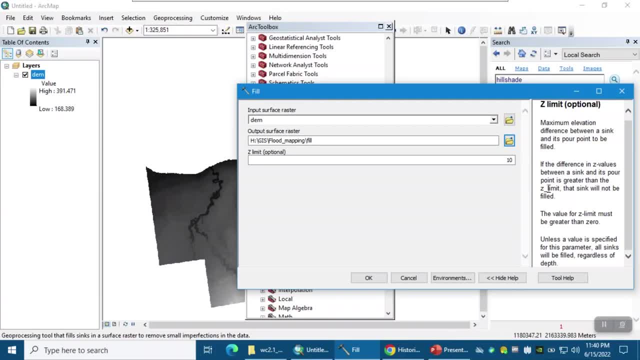 that if the difference in z values between a sync and its power point is greater than the z limit, the sync will not be filled. okay, and the value for z limit must be greater than zeros. we don't have any natural uh thing, so i'm gonna click on ok and have this: convert this digital elevation model. 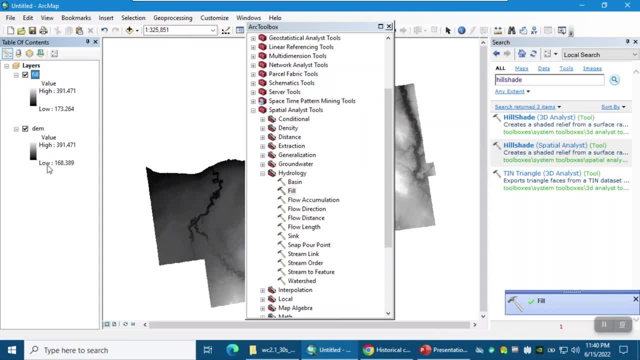 to fill it. okay, so, as you can see. uh, so the values for digital elevation model start from 168 to 391, but here, after removing the sync now, it starts from 173. so, in summary, fill function corrects your digital elevation model. okay, so sometimes fill is called depression, less digital elevation model. 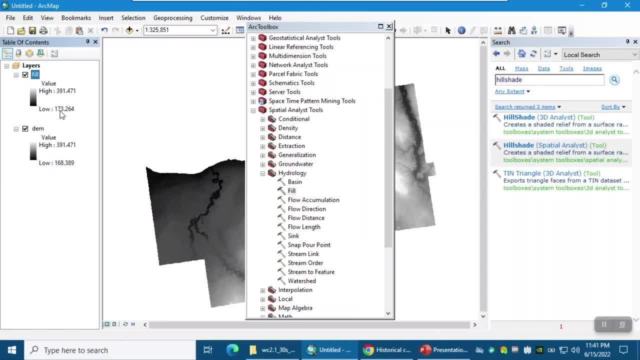 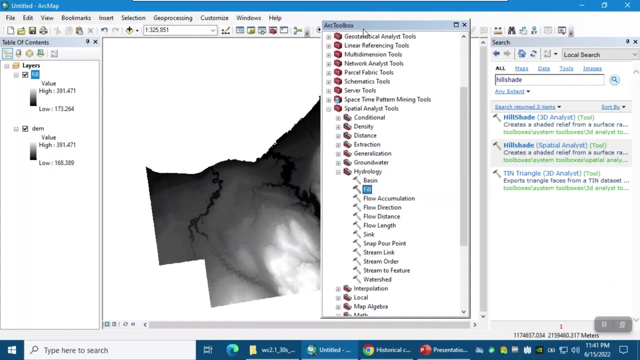 okay, so it's a corrected version of digital elevation model and then you can see um, you know, And there is a subtle difference between the digital elevation model and field, But we're going to use field for the following steps. So the next step is that we need to create flow direction raster. 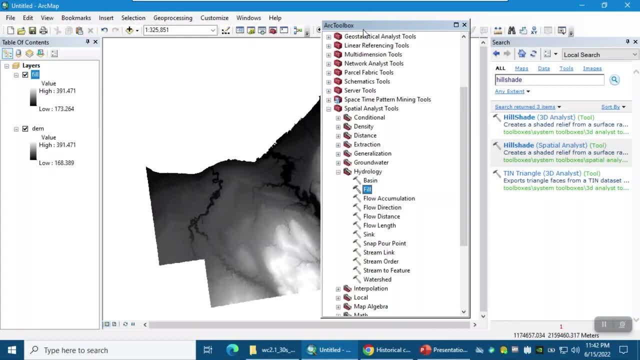 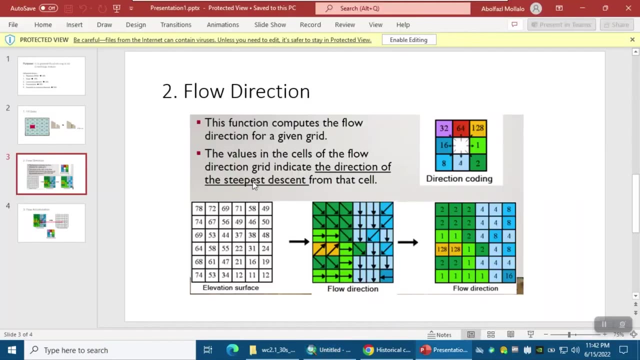 And flow direction. raster means: if rainfall falls on the surface, how would it flow? And we assume that water flows following the slope direction, In other words the direction of steepest descent, For instance in this image, these are the pixel values of digital elevation. 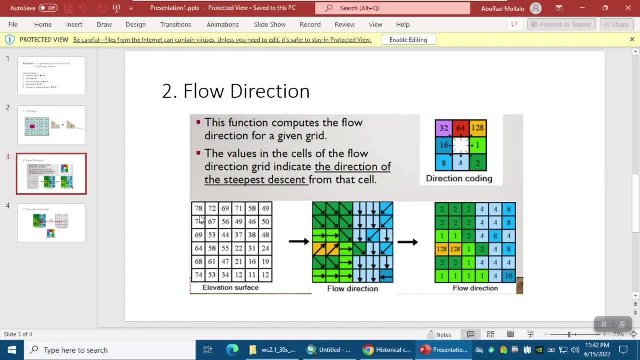 So these are the pixel values of digital elevation model. Okay, so from 78,. so which pixel or the neighbor pixel has the lowest value? So it's obviously 67. And you can see that the water flows in this direction From the second one. for the second one: 72,. 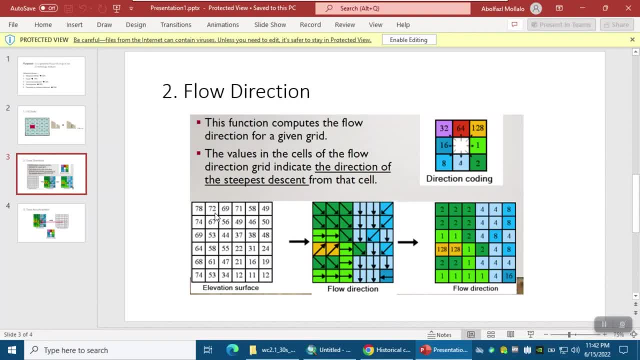 which pixel Pixel value causes the steepest slope? And definitely 56, right, So it's going to be in this direction. So that's why you can see flow direction is in this direction And for 69, it's going to be. for 49 is the cause's deepest value. 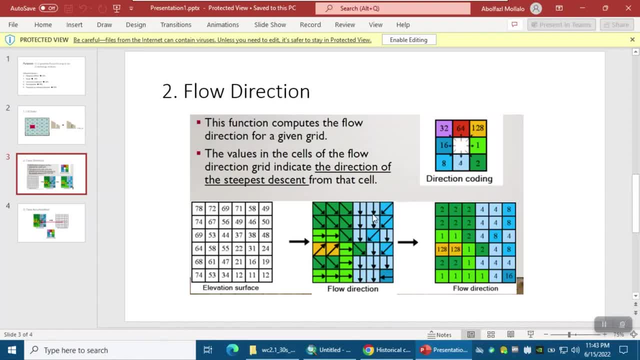 For example, 58,. this one has the lowest value, So it's in the downward direction. Okay, so this is our flow direction. But how we can? computer cannot understand the direction, Can understand only the numbers, right. So in order to recode it, we have to use this value. 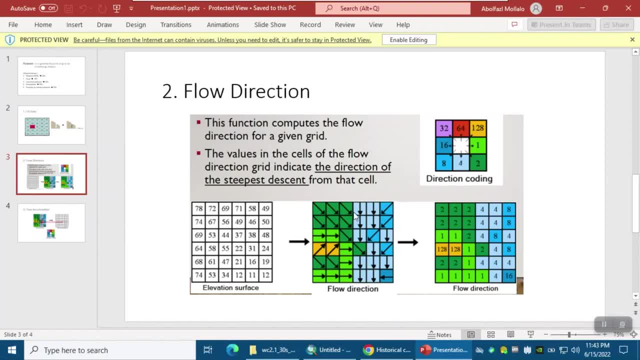 So if it's in this direction, we recode it with two. So two, two, two. If it's in the south direction, we recode it with four. If it's in this direction, we recode it with eight, and so on. 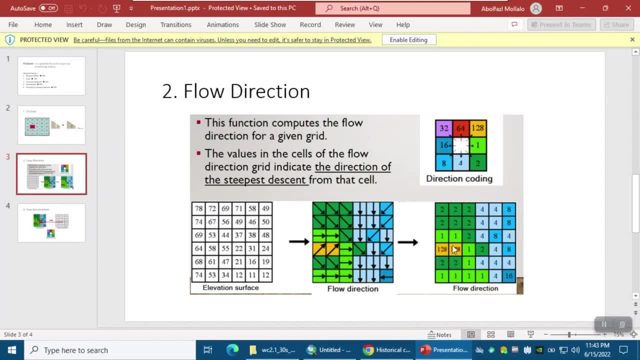 Okay, so this is going to be a so flow direction. it creates a matrix of numbers, but the numbers have a meaning. Okay, so, for example, 128 means that the direction is for the north end. Yes, direction of the. the flow direction is in the north end for for this specific cell. 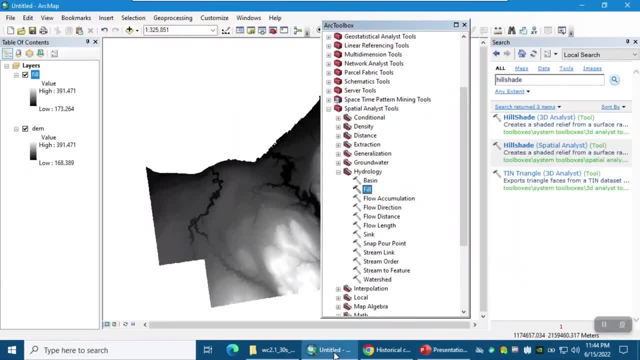 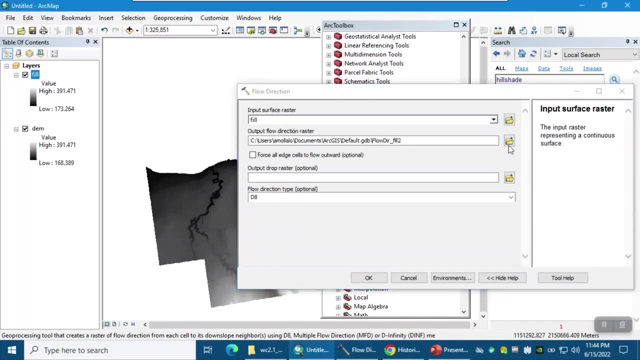 So how we can create flow direction. So we're going to create flow direction based on the field, digital elevation model. Okay, So again from hydrology, flow direction, your surface raster is going to be your field And the output raster is going to be flow. 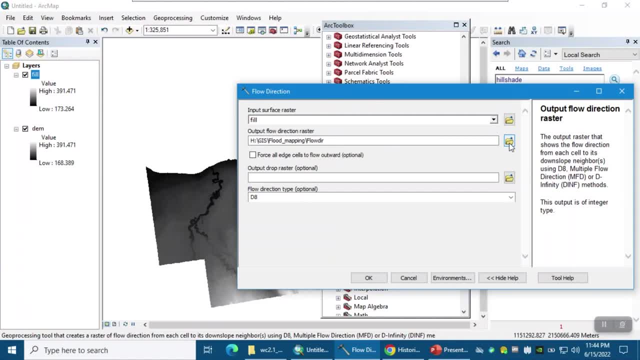 So I'm going to call it flow D I R, low direction, And we don't want to force the edge cell to flow outward. And if, uh, because in the edges the errors are very high and we don't want to involve them in our calculation. 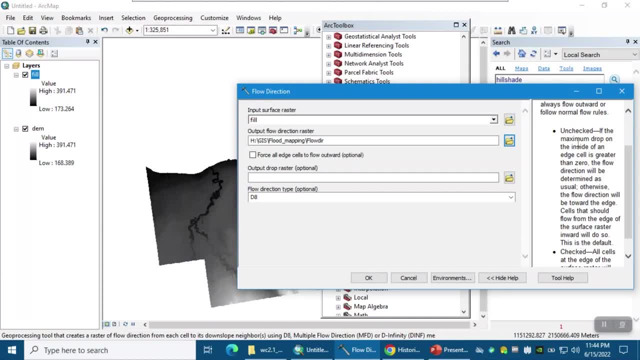 Okay, Which is the default value if it's unchecked. So, and if it's checked, uh, all cells at the edge of the surface raster will flow outward from the surface raster, And we don't want that, Right? And uh, the, the technique for flow direction type is D eight is the thing that I just explained it. 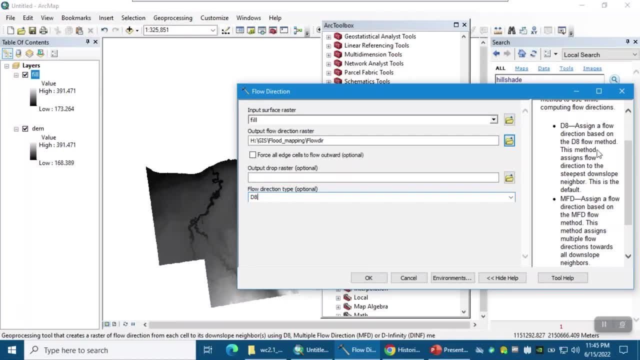 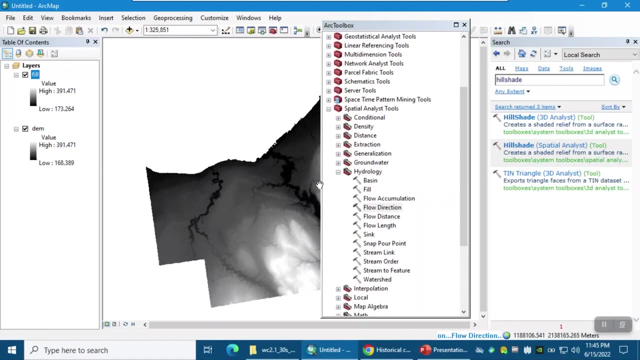 Okay, Assign a flow direction based on the met low method, And this method assigns flow direction to the steepest down slope neighbor and which is the default value. So I'm going to select D eight and click on Okay. So it creates the flow direction and the values that we can see: one, two, four, eight, 16.. 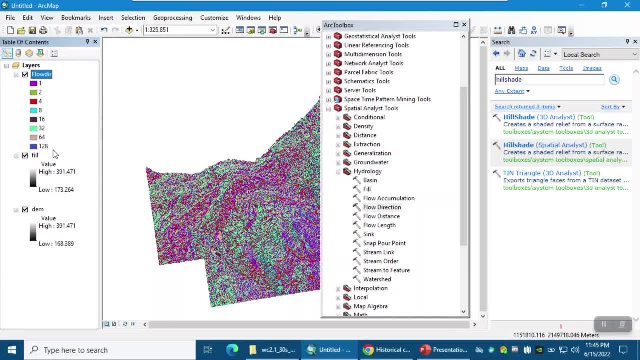 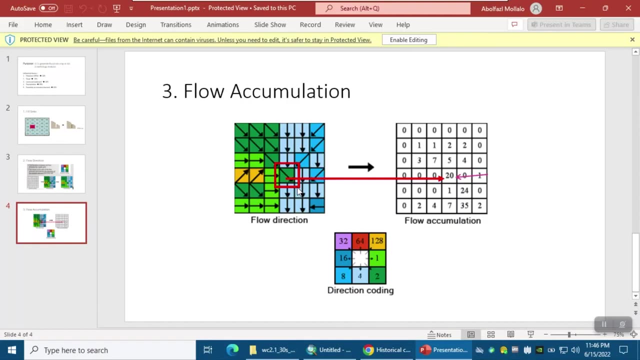 32, and so on, which I explained. what does it mean? So, after having the flow direction from the uh bill right there, the next step is to find the flow accumulation. Flow accumulation counts uh the amount of water or uh upstream cells that flow into a pixel or down a slope cell. 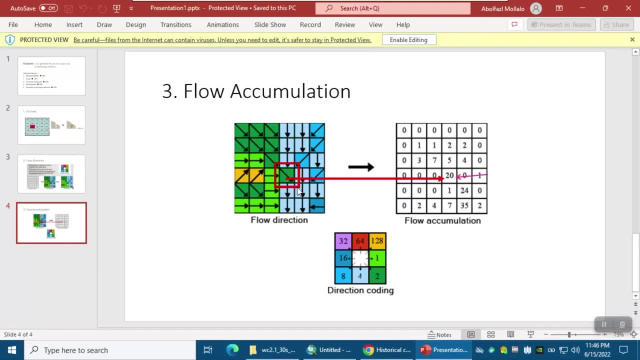 So, in other words, what is the gain of each pixel? Okay So, uh, from a small streams to larger streams and from larger stream to reverse. Okay So, to create flow, uh, accumulation, we have to use flow direction. 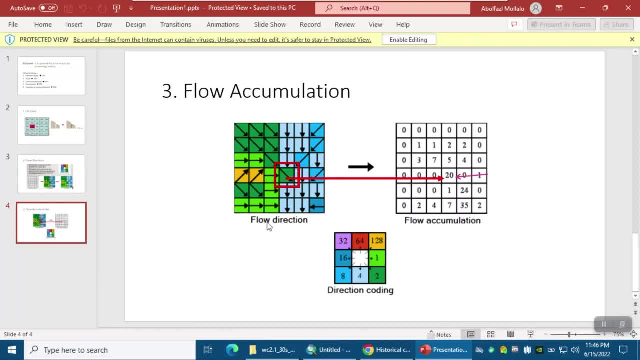 Okay, So the input for the to create a flow accumulation is flow direction And uh, for example for this one, how many units of water flow into this cell? So definitely one unit is flowing in this cell, right? That's why it is one. 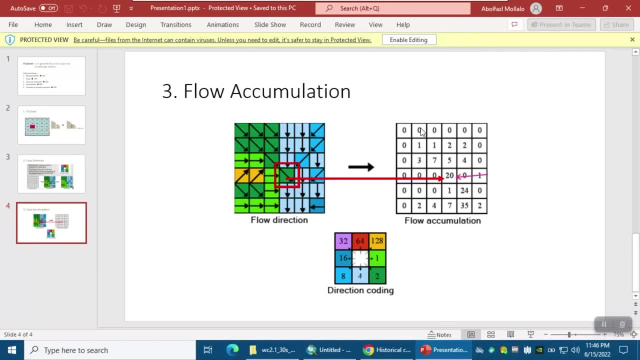 So how many, uh, how many units of water flow in this cell? Zero, Okay, But how many, uh, how many units of water flow in this cell. So this is going to be for this cell. It's going to be one, two and three, right? 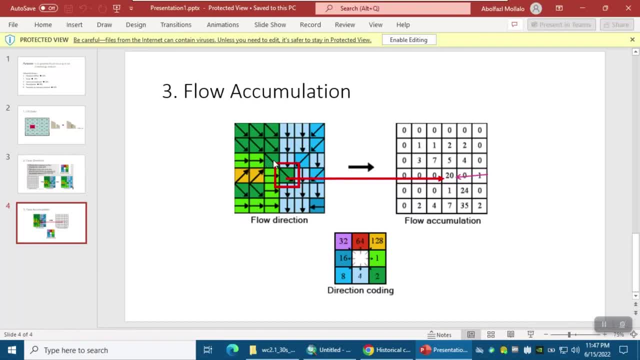 So that's why it is three, So why this pixel gets the value of seven, One, two, three pixels, uh, or unit of water flow in this cell right. And another thing is that they already have the value. They already have the value of one, three and zero. 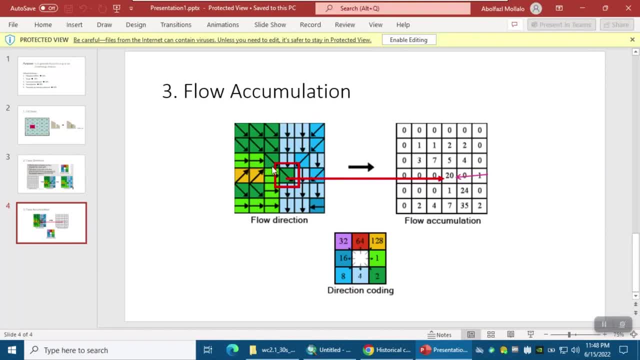 So it's going to be one plus two. one plus one plus one is three plus one is four, plus three is seven, plus zero is seven. That's why this cell gets the value of seven. So keep in mind that each contributing cell has a gain from others and also from rainfall. 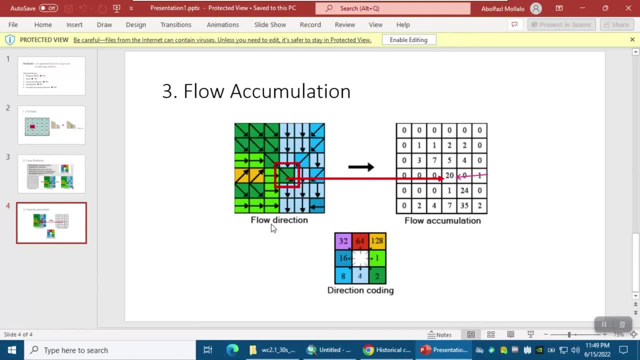 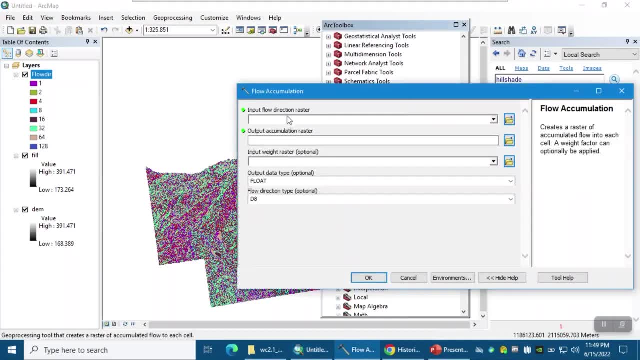 So that's how the flow accumulation can be calculated from the flow direction. Okay, So again from uh ArcMap, if you click on flow accumulation, so the input is going to be your flow direction raster, So it's going to be flow direction raster. 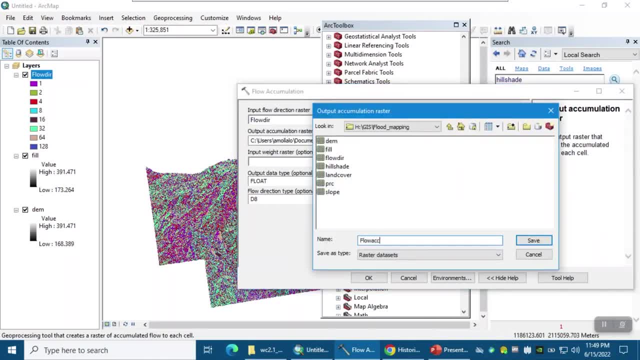 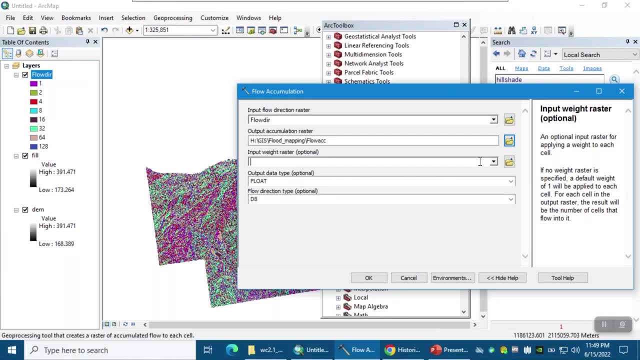 The output is going to be flow ACC, flow accumulation. So, uh, we don't want to apply weight uh to each cell and the result is based only on the number of cells that flow into that specific cell. Okay, So, uh, we accept the. 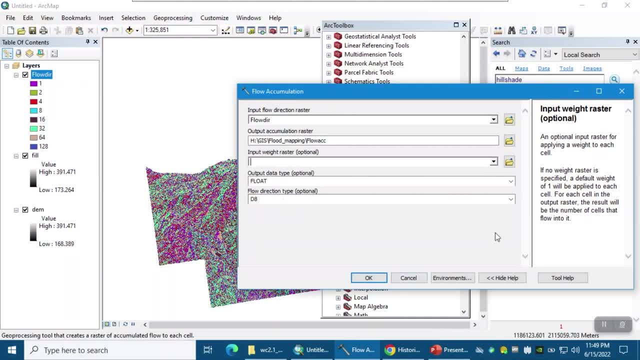 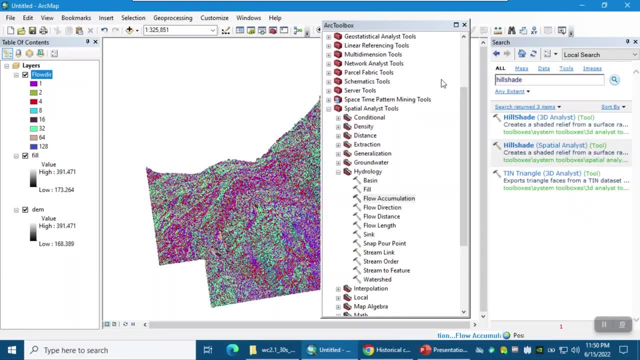 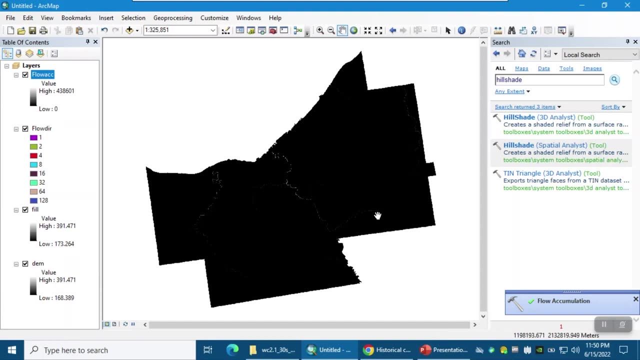 Other. so, for example, flow direction type is D8 and so on. So we accept the other uh default settings and click okay, All right. So here is the result of flow accumulation. So uh, the pixel values, if you use identify button here. so the pixel values, for example, here is zero, here is 29,, here is zero 38.. 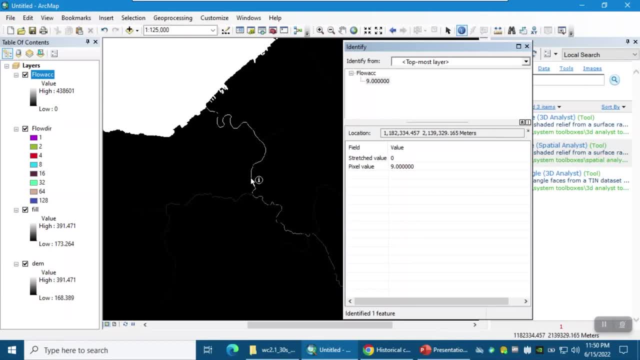 Okay So the pixel values shows the number of cell upstream that flow in that cell that we just discussed. Okay So the cells with high flow accumulations should be in lower elevations, such as in valleys or drainage channels. Okay So this image is kind of very dark. 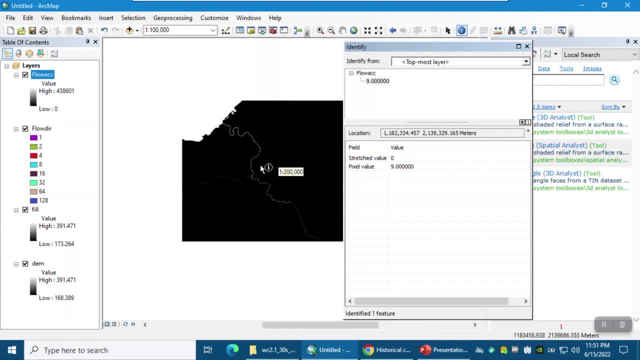 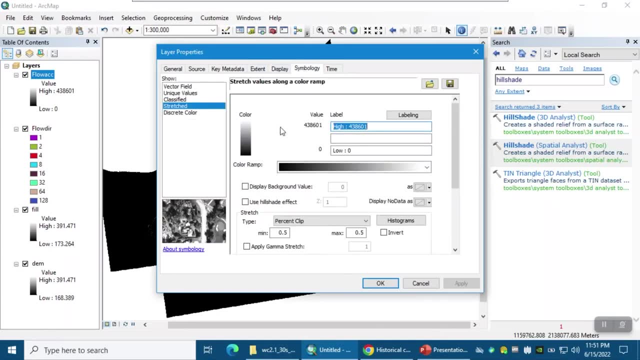 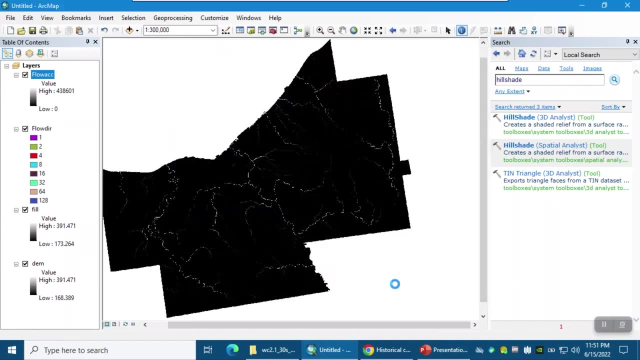 So, uh, but uh, you may see the streams. right, You can see the stream, But let me change the symbology of this layer. So if I go to the properties of the flow, accumulation Symbology, and here uh, stretch it based on the uh standard deviation and then apply an, okay, 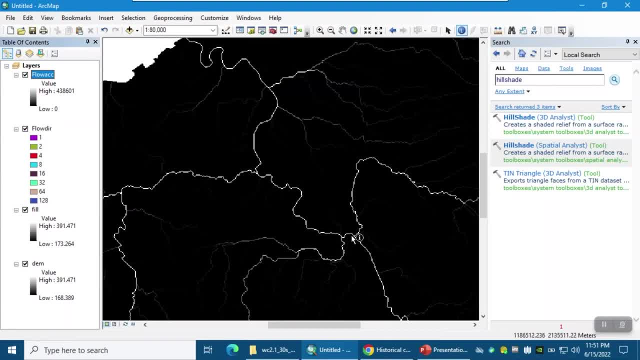 So here you can better see the channel stream of uh streams or channels based on the digital elevation model. Okay, So, as you can see, some streams are main which have the higher uh values of the flow accumulation, and some of them are not main channels. 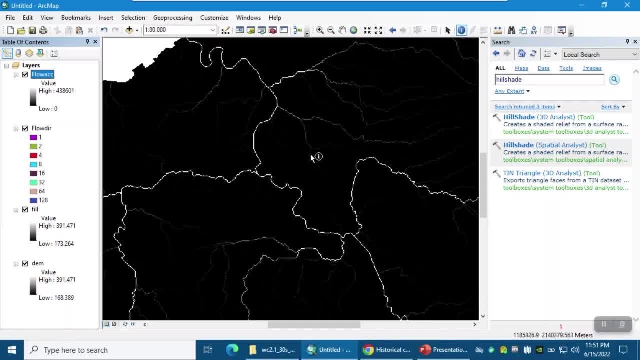 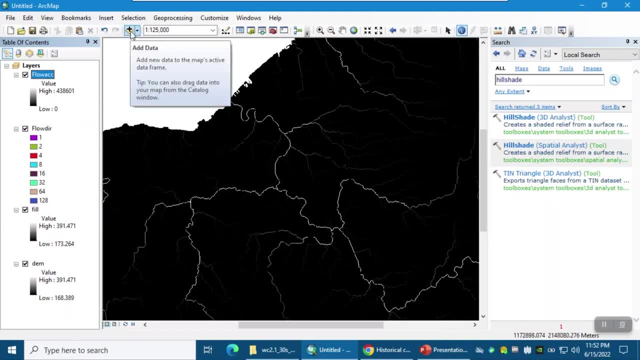 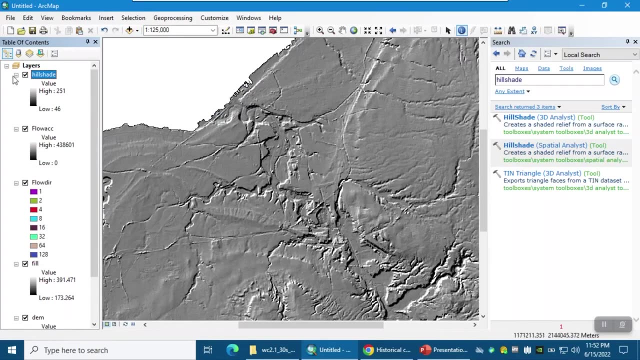 Okay, So we're going to, So we're going to- focus on most on the main channels or main streams. Another thing is that you can compare this streams with the hill shape that we just created. So if you look at the hill shade and add it here so you can see that. 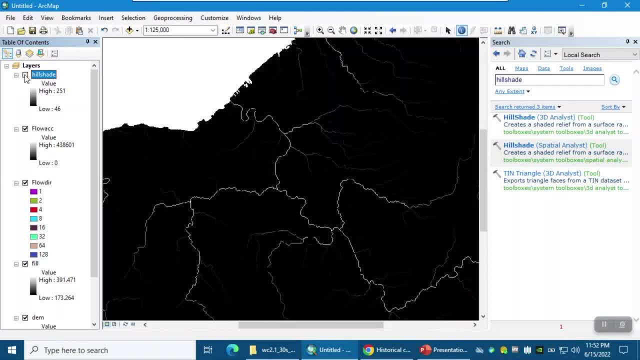 So it's, it's kinda, uh, so this flow accumulation is kind of identified: the hill shade right, So, uh, the channels or streams that are visible, Okay, So let's go from the hill shift, So let me remove this hill shade and we're going to focus on this flow accumulation. raster grid. 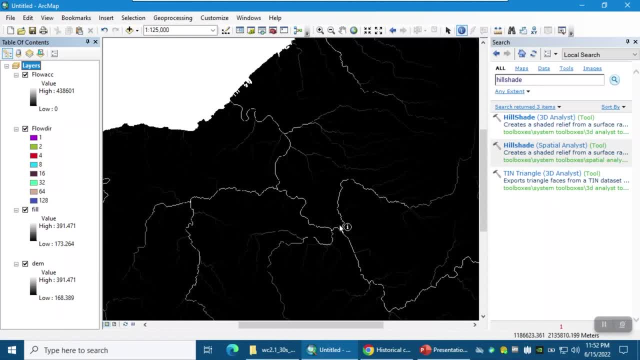 We would like to extract the stream, channel uh, from this raster grid And if this Dell value is greater than a threshold, we're going to assign it to to a value of one which, because it shows the main stream, And if the cell value is not greater than the threshold, 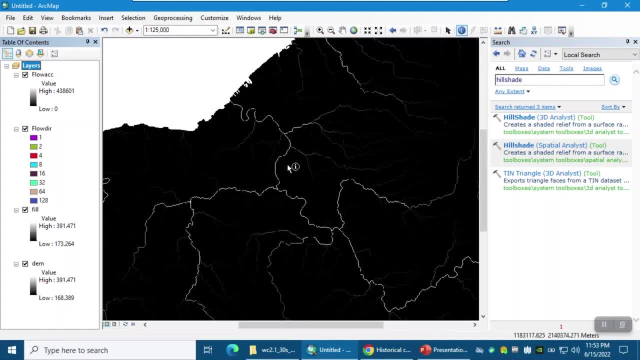 You have to assign it No data. Okay, So it's going to be one or just a stream or no data, And a rule of some for a stream threshold is that the threshold is 1% of maximum flow accumulation. Okay, So the maximum flow accumulation is 40,- uh, 438.. 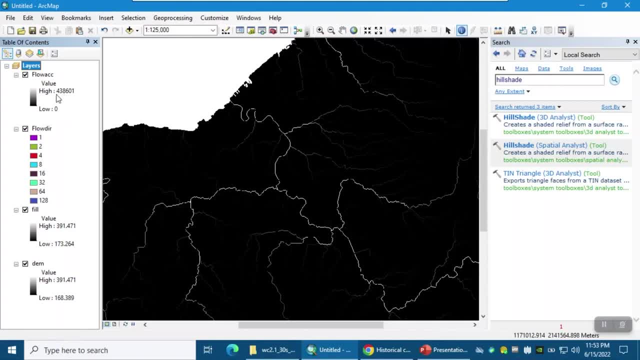 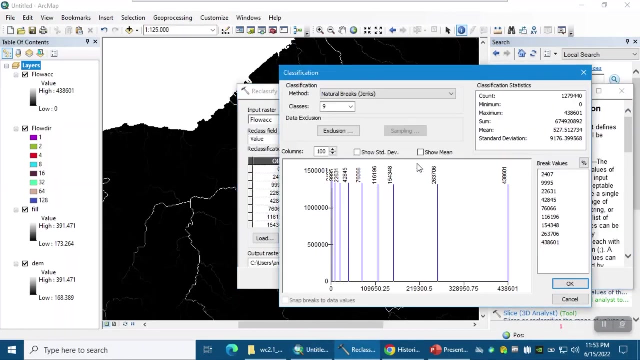 So the threshold that I'm going to set is like 4,400.. Okay, So it's 1% of the maximum flow accumulation. So I'm going to Reclassify this raster. So if I type, reclassify uh into two classes, so for the flow accumulation I'm going to reclassify it into two classes. 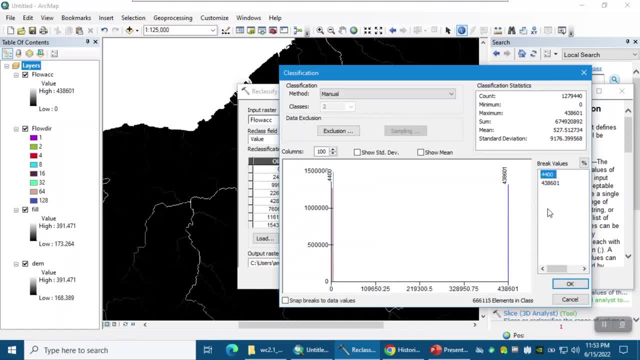 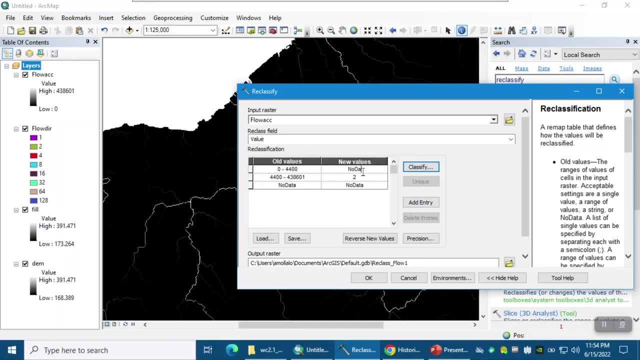 The value is going to be 4,400 and anything after that is going to be one. So this is going to be no data, and here make sure that D is capital and Anything above the threshold is going to be one, because it shows the main streams. 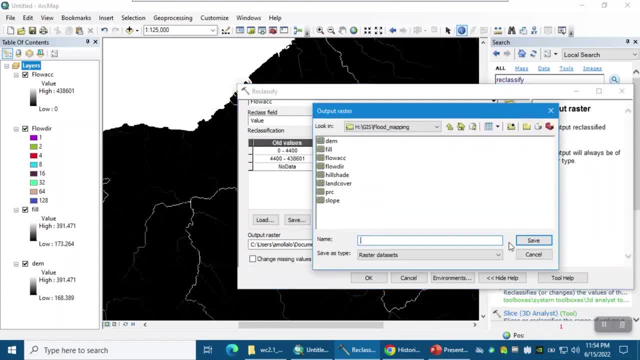 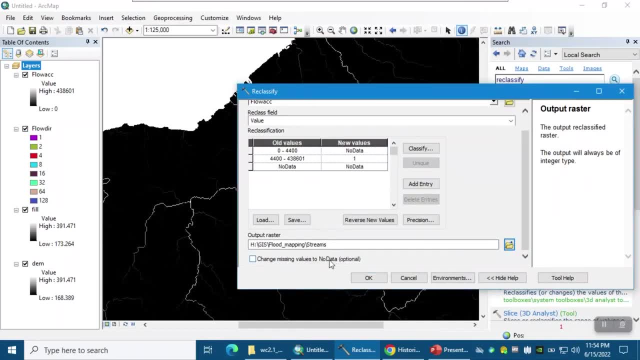 So these are the flow accumulation and, uh, the output is going to be our streams. Okay, So this is how we can extract the streams from the digital elevation model and, Uh, change missing values to no data. So let's click. 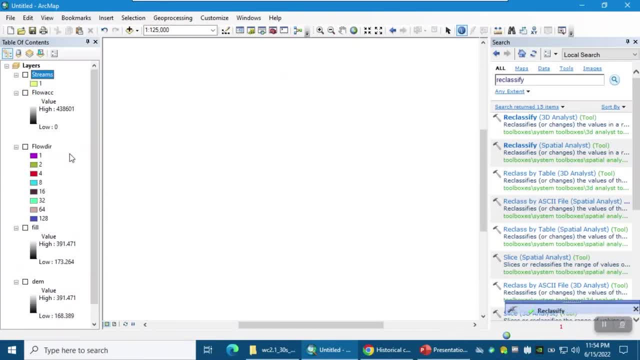 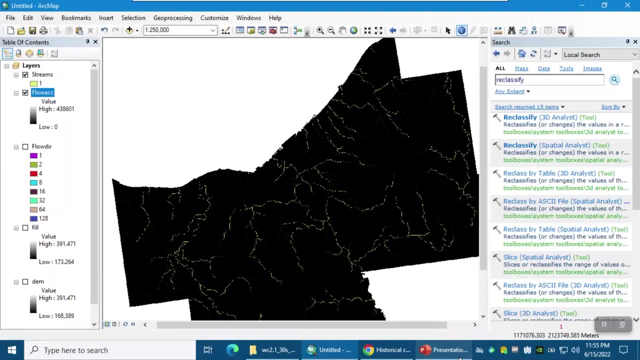 Okay, Turn on layer off, and here we can see that. So these are the streams that we detected that from The digital elevation model. Okay, So, uh, I just wanted to show you the application of hydrology extension so you can also delineate water fed and also use it in utility network in the future. 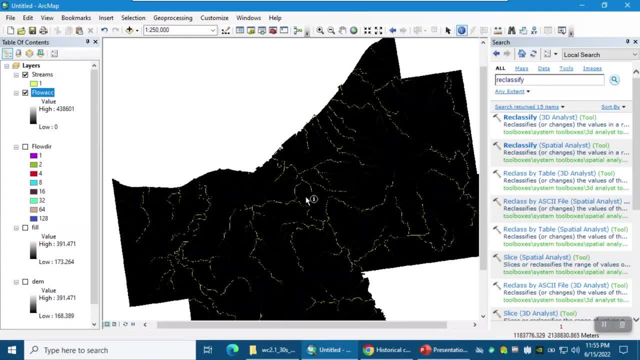 All right. So we found the streams from digital elevation model based on multiple steps that we took, but we need to find the proximity to these streams or channels. Okay, And the function that you know is Euclidean This Okay, So if you type Euclidean and Euclidean distance, spatial analyst, so we're going to find the distance to this streams. 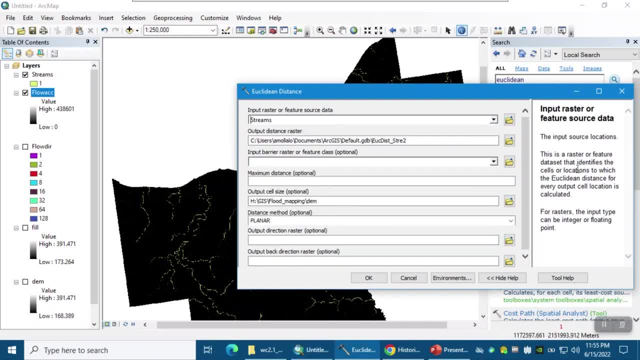 Okay. So your input is going to be a streams, and uh, because we don't need to convert this to the feature, or uh, polyline, because it also can get the raster. Okay, And um, also the outputs. So this is a raster or feature data that identifies cell or location to which the Euclidean 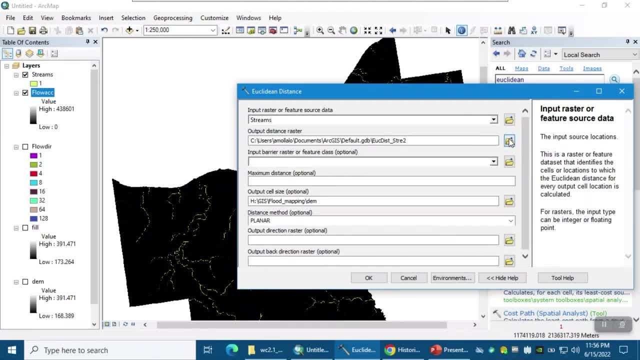 Distance is calculated. Output is going to be uh. okay, So what is the output? The output is going to be: for each cell in the output, the Euclidean distance uh to the closest cell uh will be calculated. 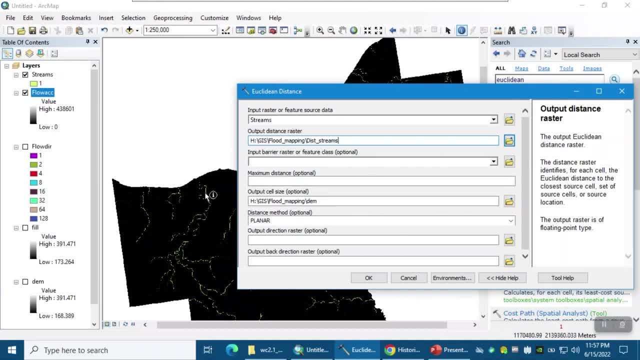 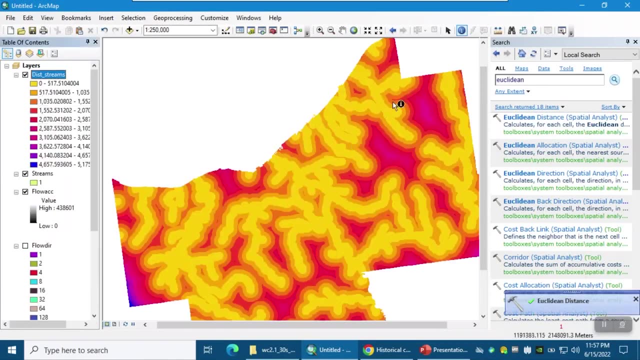 Okay, So it's going to be the distance. distance to this stream, Okay, And uh, what else? The cell size is like the digital elevation model. Everything is good And then click okay, All right, So, as you can see. so these are the distance to the streams or the channels. 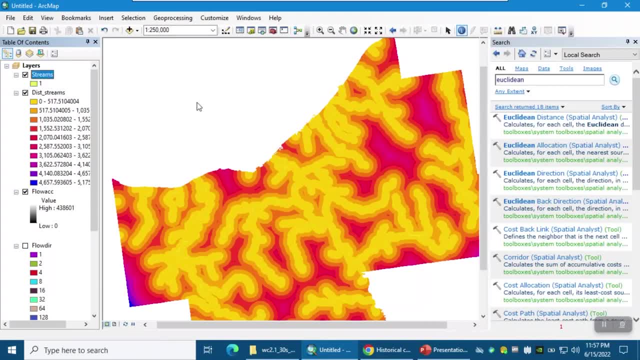 Okay, So when you are closer to the stream, when you are closer to the stream, the distance is lower. When you are far from the streams, the distance is going to be higher. So that's the proximity to the streams or channels. 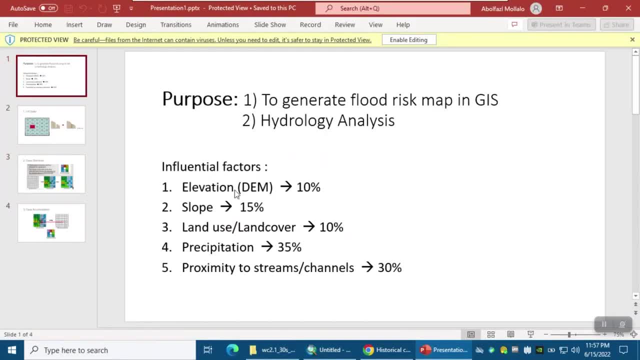 All right. So we have all the information right. We have elevation slope, land Use, Land cover, precipitation and then proximity to a streams. So what is the next step? Let's only keep the uh stream distance to a stream layer or proximity to a stream. 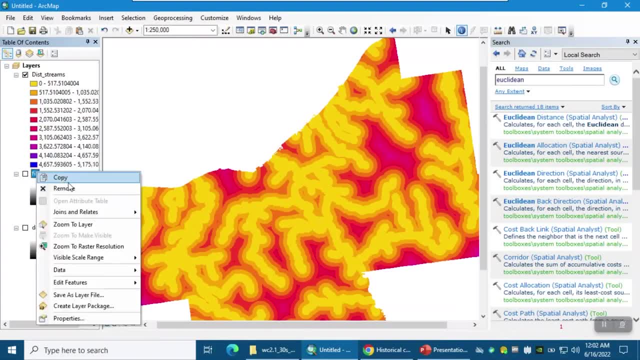 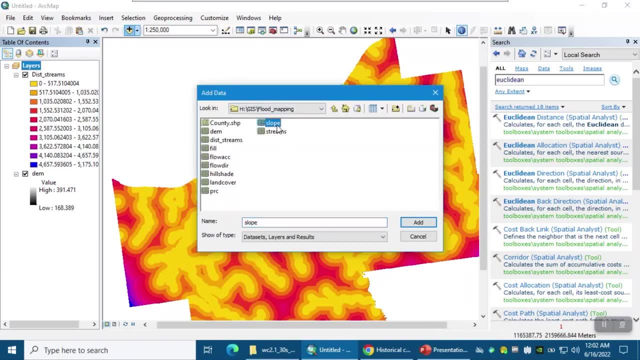 So we don't need the flow accumulation, We don't need flow direction, We don't need fill, We just want to have digital elevation model. We have proximity to streams, We need a slope, We need county, and then land cover and precipitation. 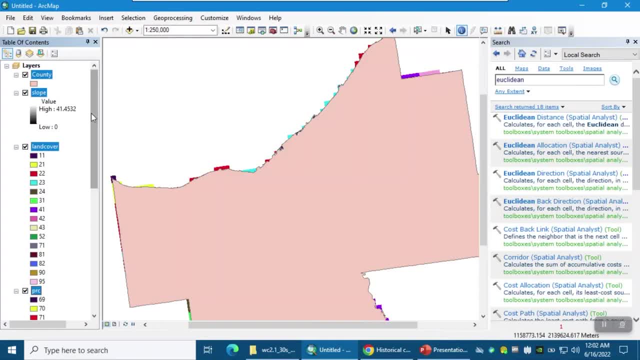 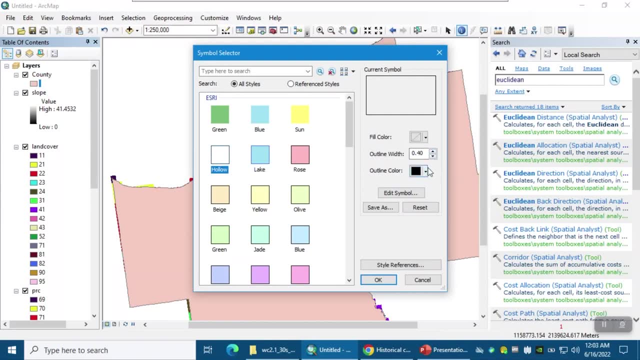 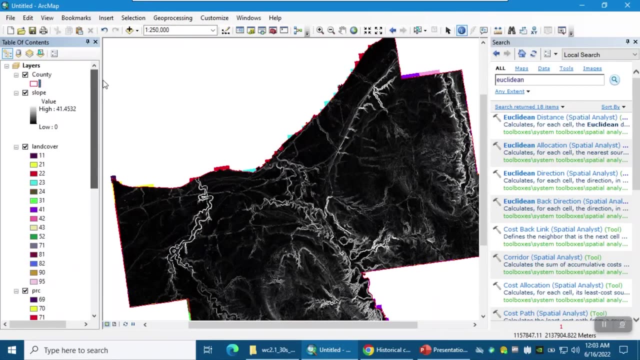 So this is where the Okay Uh factors that we need it right. So for the counties, we are just need to have the uh hollow and uh red color for the borders. Okay, So this is uh, these are the variables that we're going to focus on. 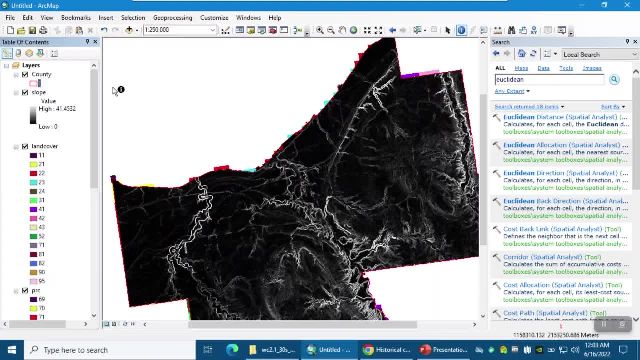 So, similar to the suitability analysis lab, we need to reclassify all layers uh, which makes them all unit lists and ready for overlay analysis. Okay, So we have to reclassify them into the common scale that uh zero means not suitable. 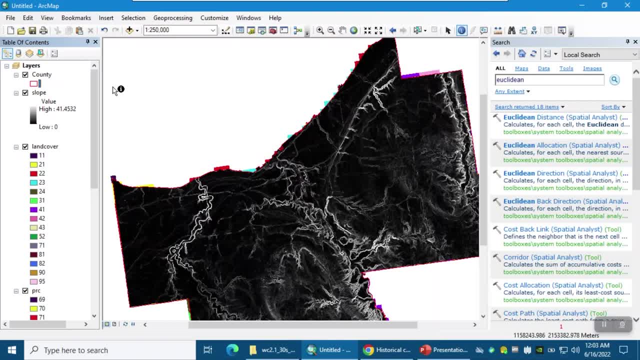 Two means very low, four means low, six means medium, eight means high and 10 means very high suitability. Okay, So the first one is digital elevation model. Okay, So we have to reclassify, uh, digital elevation model. 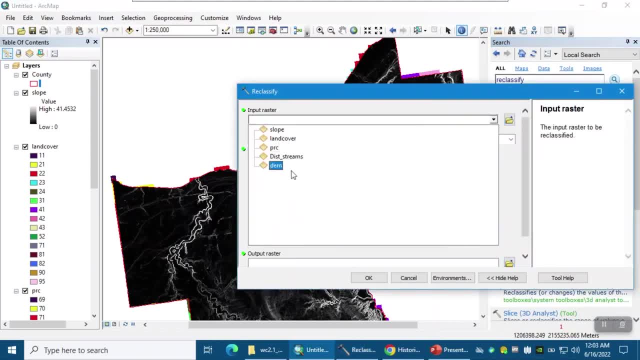 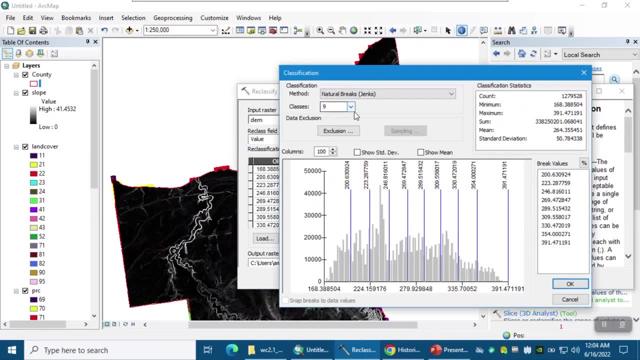 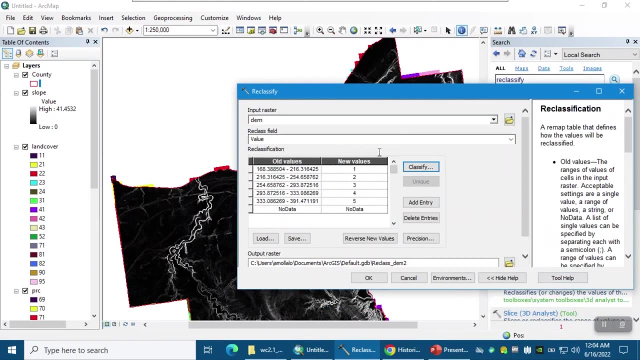 So if you select reclassify spatial analyst And focus on digital elevation model, click on classify- So uh, we're going to have five classes based on the natural break classification technique and then click Okay, So uh, it is obvious that the flat areas are more at risk of flooding compared to the regions with a higher elevation. 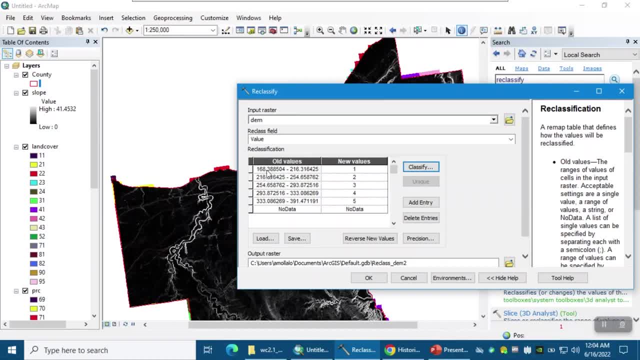 Right, So for the, for the first one. so these are the flat areas. So it It is the high risk area. Okay, So we're going to create the map of flood risk. Okay, So here is going to get the value of 10, which means that high, very high suitability for our floods. 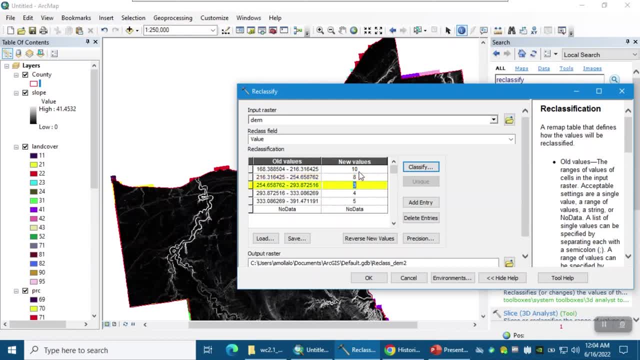 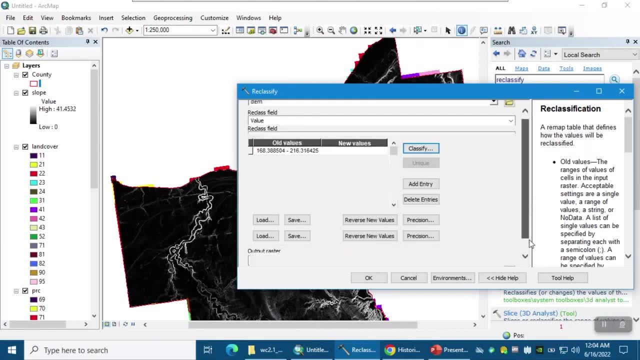 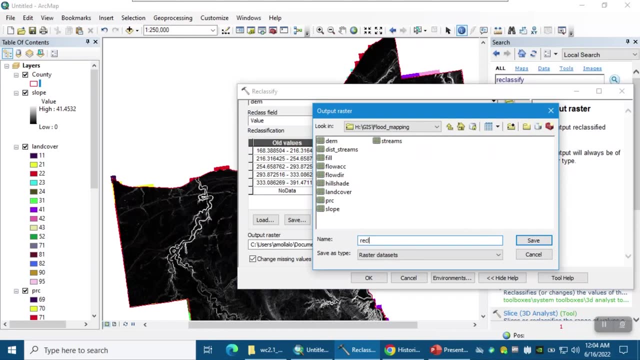 Okay, And then eight high, six, four and two very low suitability for risk, And we're gonna uh, also change missing values to no data And the output is going to be reclassified And, uh, we have the class of digital elevation model. 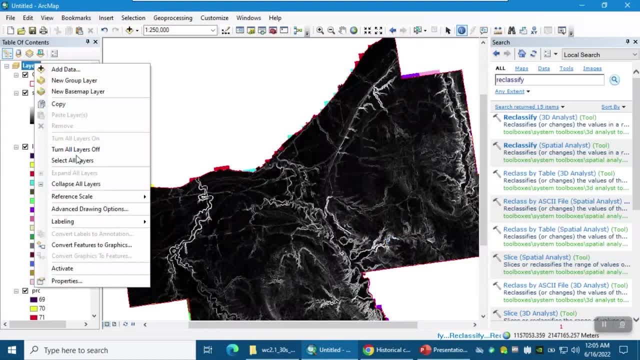 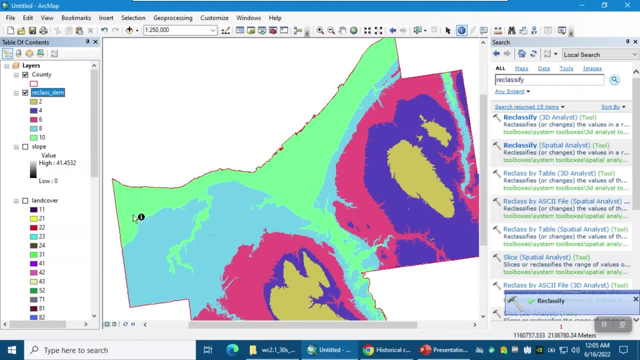 Anything else and click Okay, So let me turn on layer off. So here you can see that. So when you are so here, when you are closer to the low land areas, closer to the lake, we have the highest suitability for flood, which kind of makes sense. 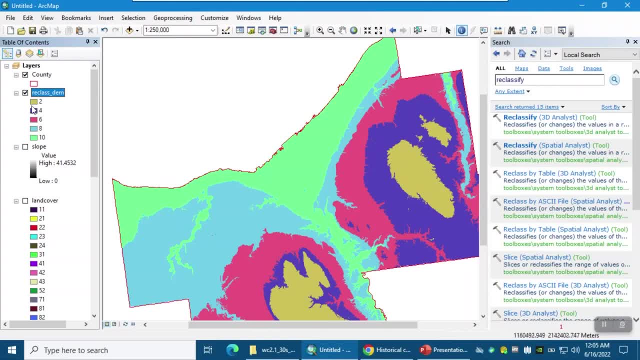 And In these areas with that are very high elevation, We have for flood All right. so the next one is a slope and, similar to a digital elevation model, flat areas or lower slopes are more flood prone because lower slopes increases the quantity. 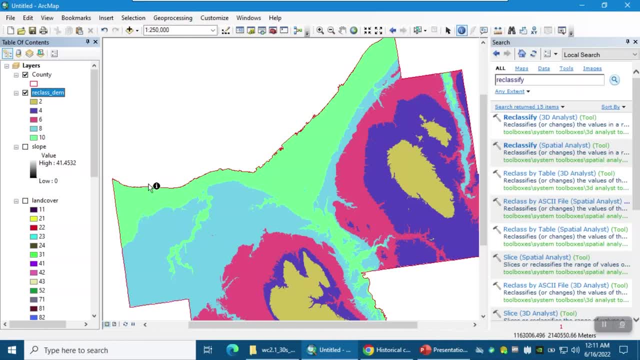 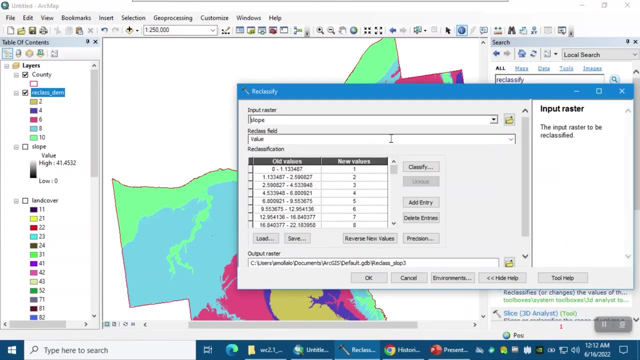 of water soaked into soil right. So lower elevation and lower slopes are more susceptible to floods. So again from reclassify: if you select spatial analyst and then here, based on this slope, I'm gonna reclassify it into click on classify. 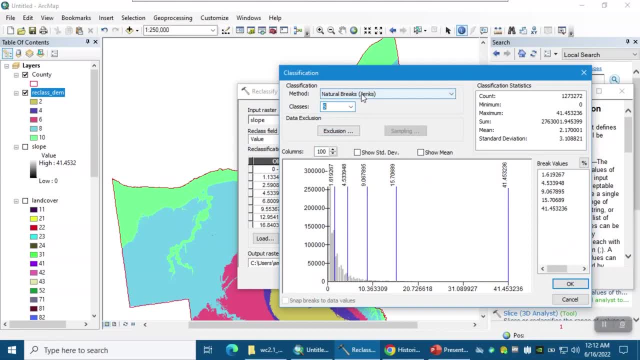 I'm gonna reclassify it into five categories based on natural break. but I'm not gonna use the natural break, I'm gonna use manual classification. I'm gonna say less than five, or sorry, less than two is very high flood prone areas right. 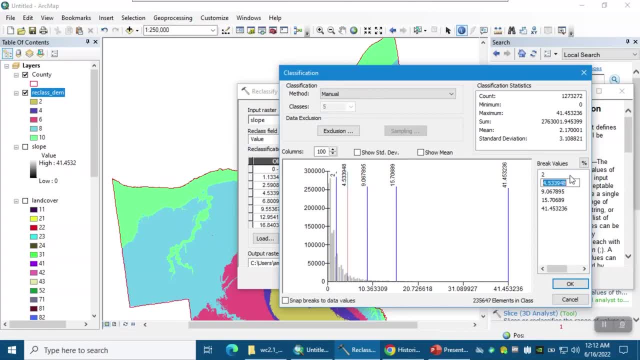 So I'm gonna select two. the next one is between two and five is high. between five and 10 is gonna be medium, between 10 and 20 is gonna be low and above 20 is gonna be very low, okay. 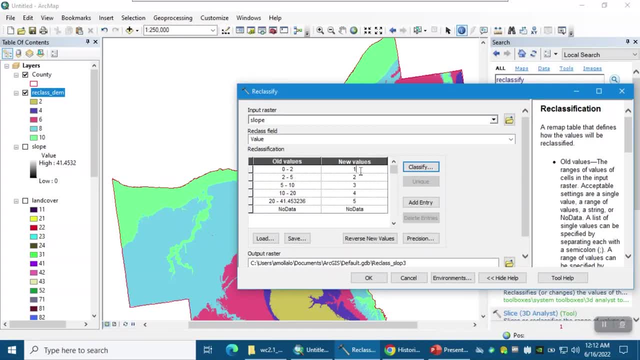 So click, okay. So between zero and two flat areas are at the highest, very high risk, right? So this one gets the value of 10, then eight, six, four and two And the output is gonna be reclass underscore slope. 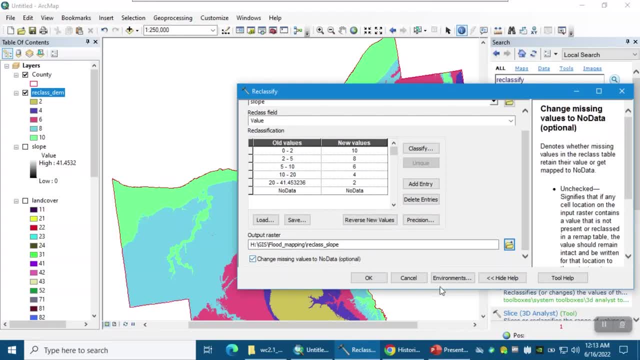 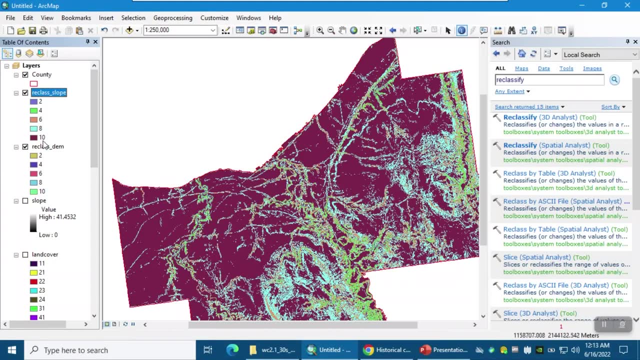 And you want to change in the same values to noted. Okay, click, okay. So, in terms of a slope, most part of this study area is like 10, it gets a value of 10, which means that they are at very high risk. 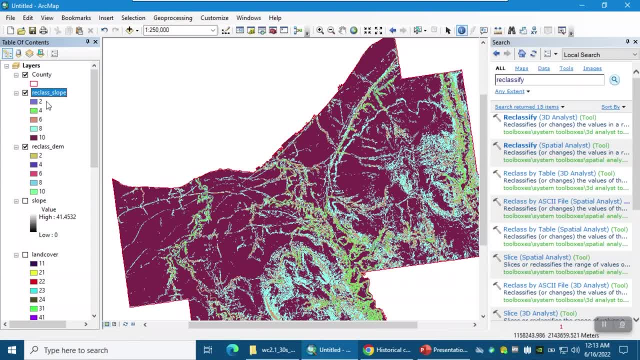 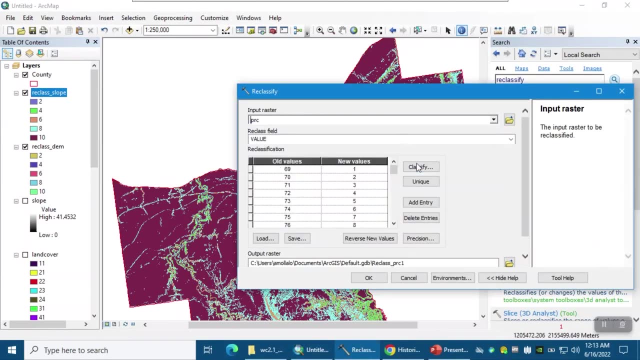 of flat, because it's kind of flat. So less than two degree slope. So the next one is precipitation, right? So again, if you go to the Reclassify spatial analyst and then precipitation, PRC, So we're gonna classify into 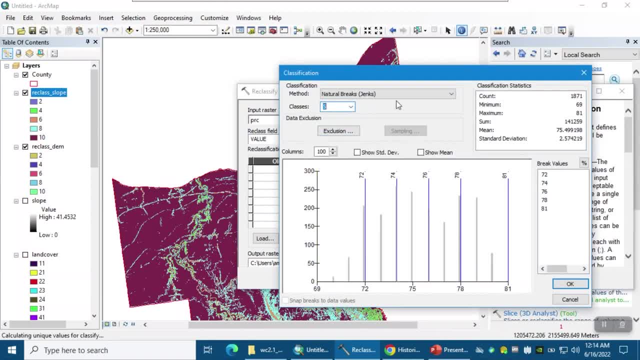 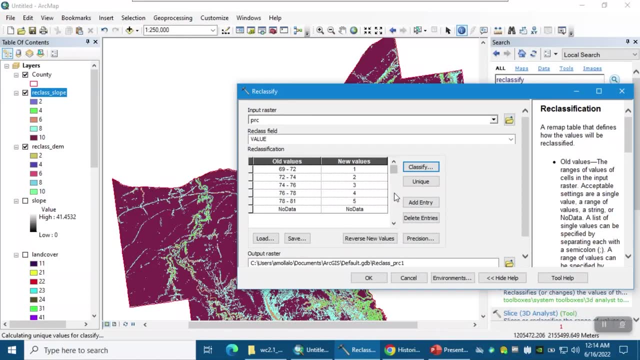 based on natural break, five classes and the output. So it is evident that the heavier precipitation intensity increases the chance of flood. right So it is a no brainer. So here it's gonna be very low importance, right So it gets the value of two. 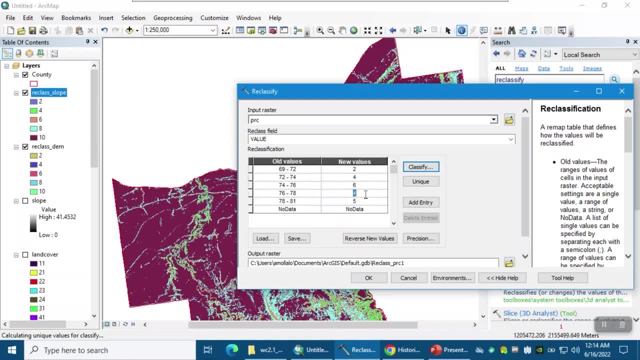 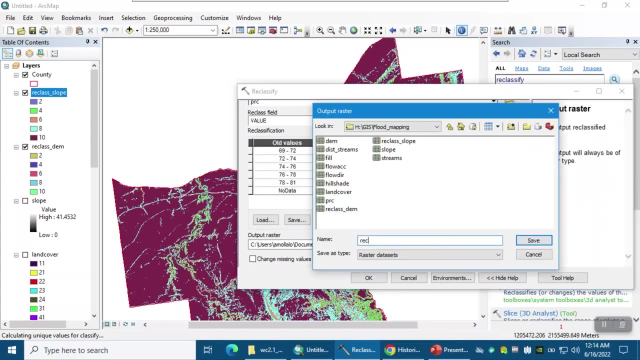 and then gets the value of four, six, eight, And this area with heavy precipitation gets the highest chance of flood right. So, or gets the highest chance of flood And that's the highest score for flood, And then here I'm gonna call it the output. 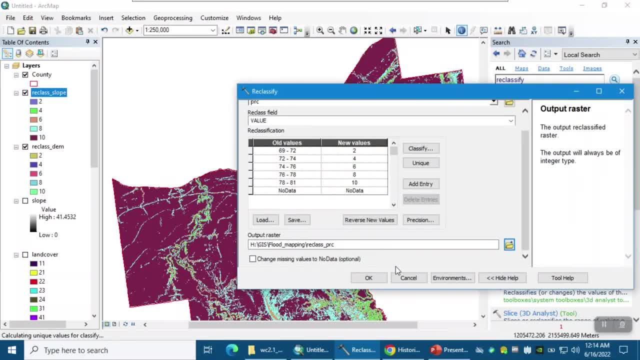 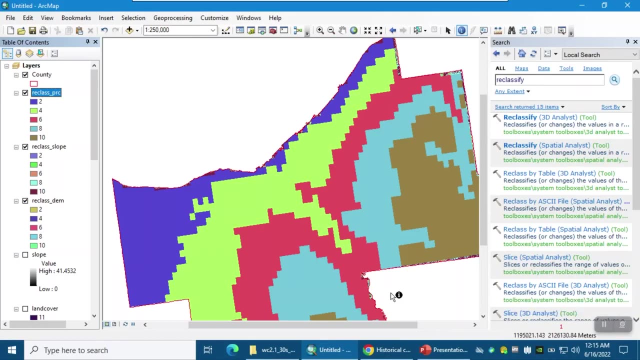 as the class PRC precipitation, which includes rainfall, melting snows and also ice and so on. So change missing values to no data and then okay, All right. so the next one is land cover, And for land cover, it is obvious that urbanized areas. 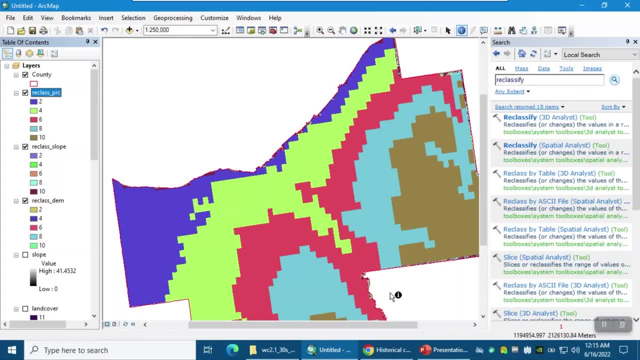 are less vulnerable than wetland areas, So this is the next one, This is the next one, So this is the next one, So this is the next one, So this is the next one, or reverse, right? so, uh, first of all, wetland areas. if you look at the legend of the land cover, so let 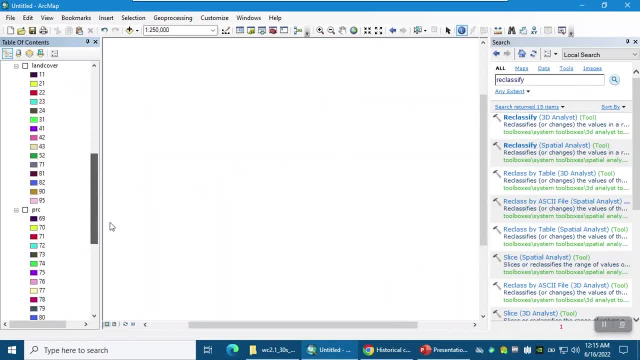 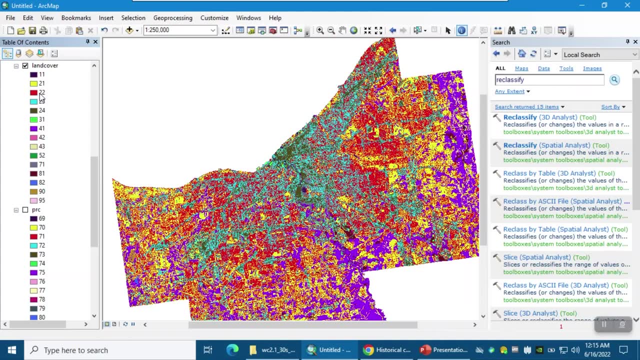 me turn all layer off for the land cover type. so the legend, the value, that is 21, 22, 23, 24 are developed areas, so they are at the lowest risk of flood right, so they get the value of two, which means that very low uh risk of flood. so the way that it works is uh if you click on the classify. 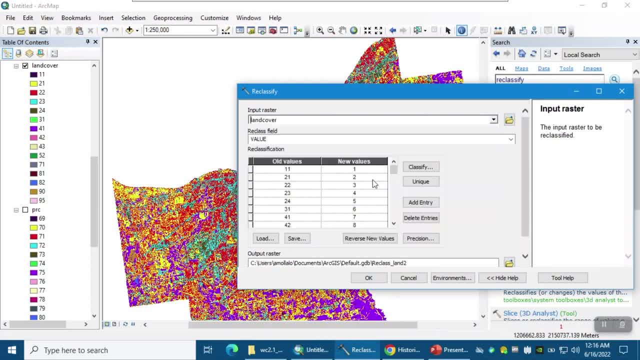 and then uh for the land cover. so for the land cover you have to click on the unique value because we're going to get all of the unique value. so 11 was open water and gets the highest value, which was uh. 10 and 21, 22, 23, 24- according to the legend, are developed urbanized areas right? 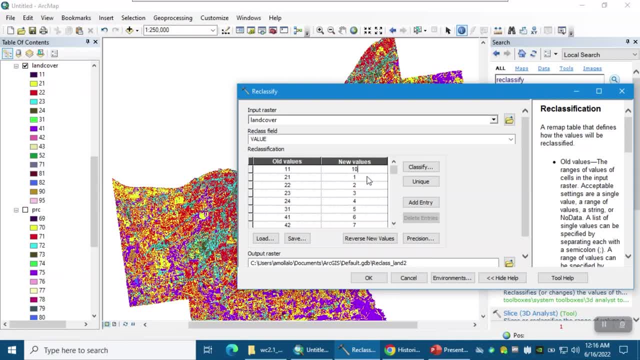 so high and this high intensity, low intensity, medium and open space. so this value, these categories get the value of two very low uh chance for floods: 24.. 31 uh 30, 41, 42, 43, 52, 71. so these are deciduous forest, evergreen, mixed forest, barren grassland, so they are in very 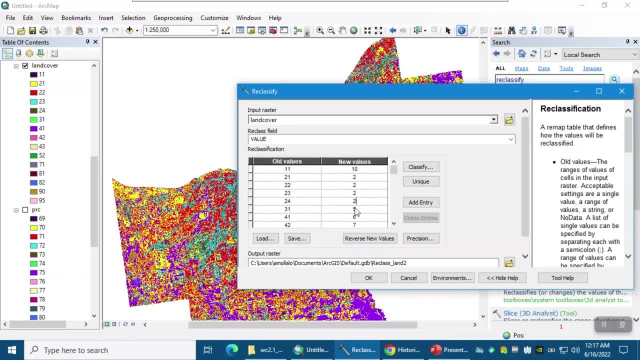 low, uh, not very low. they are low, uh, chance for chance or risk for flood. okay, so they get the value of four. so 31 is gonna be four, 41, the same for 41, 42, 43, uh, 52 and 70, 52 and 71. they get the. 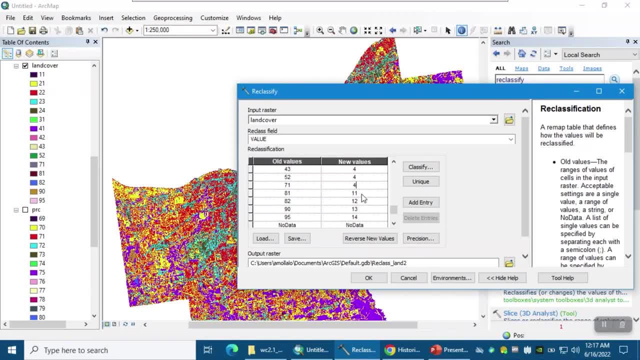 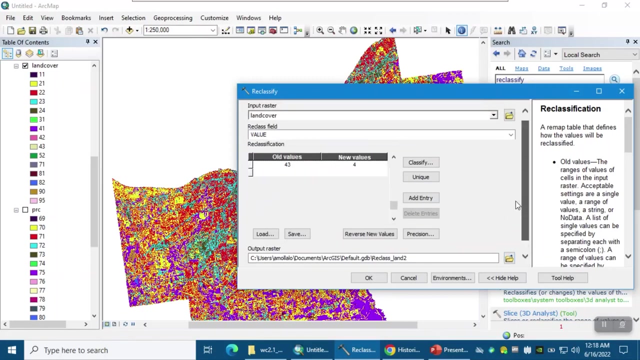 value of four. so 81 and 82 are planted or cultivated crops, so they get the value of six. and 90 and 95 are wetland areas and they are at high risk of flood, so they get the value of eight. all right, so this is how we can reclassify the raster and after that, so let me check. 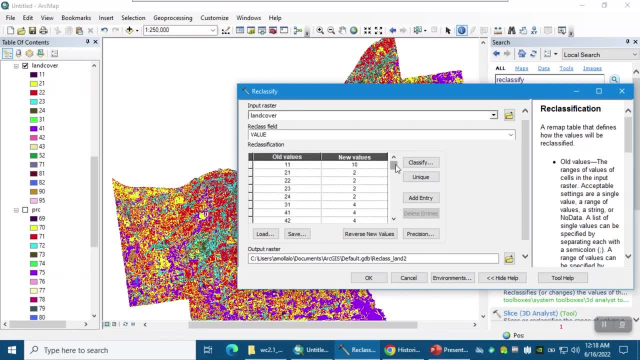 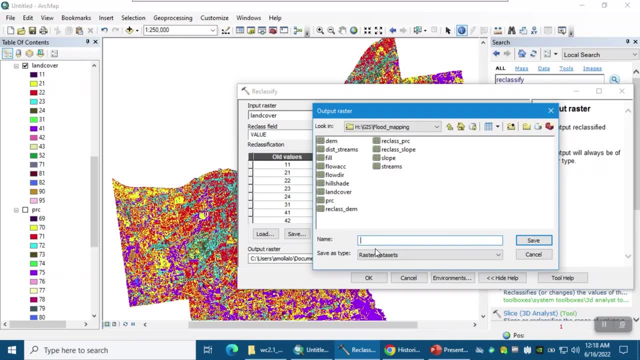 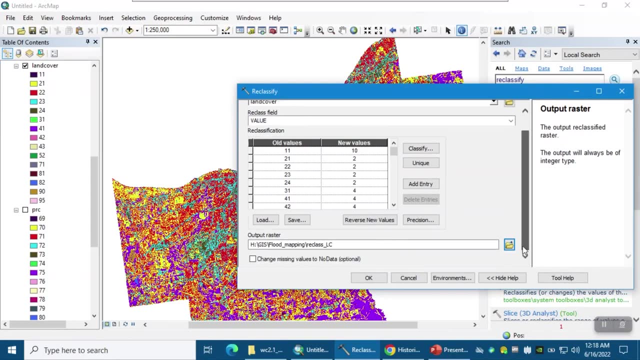 Mann, let me start with the first. one gets the value 10, 2, 2, 2, 4, 6, 8 and 8. all right, so this is going to be: reclass underscore, lens cover and change the missing value to no data, and then 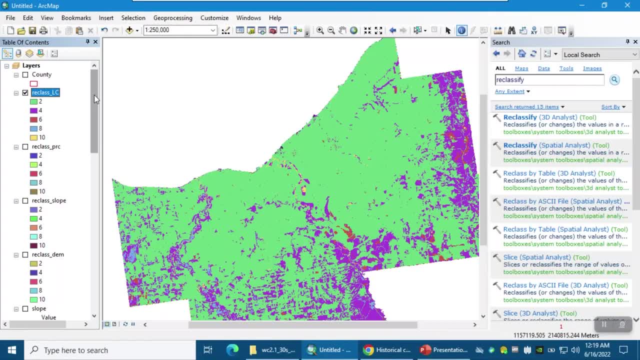 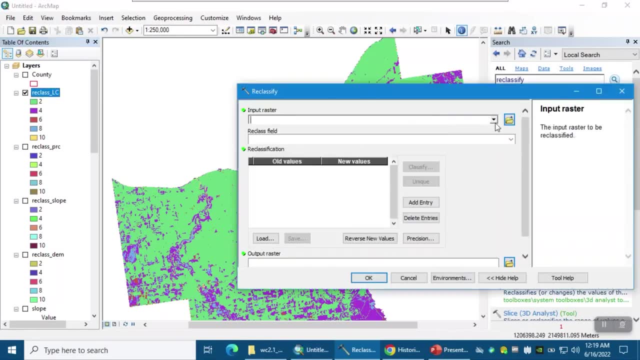 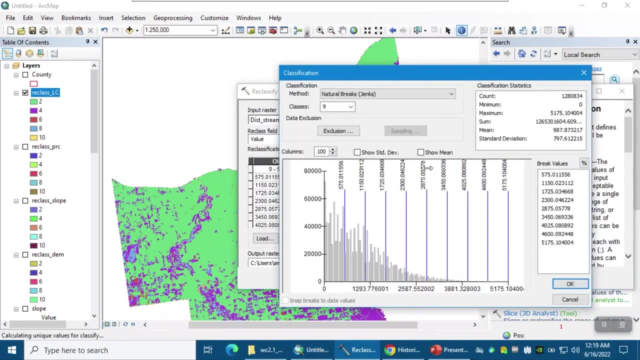 okay, all right. so the last one is proximity to streams or channels. closer distance to the streams, the higher probability for flood, right. So if you go to the Reclassify Spatial Analyst, so proximity distance to the streams and here click on Classify, 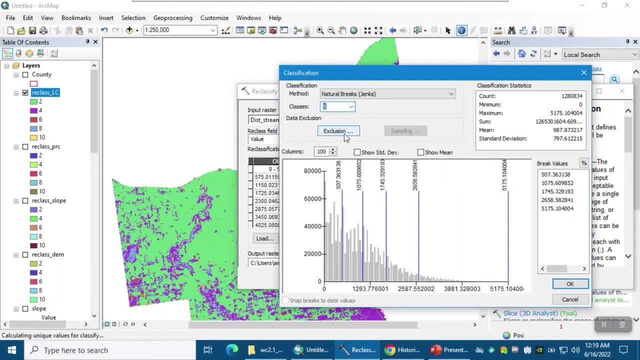 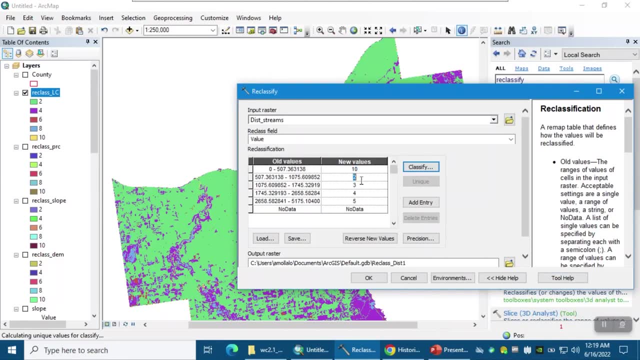 We're gonna classify it into five categories based on natural break, and then click OK, So the closer gets the highest value, So it's gonna be 10, and then eight, then six, four and finally two And after that. so this is gonna be reclass underscore. 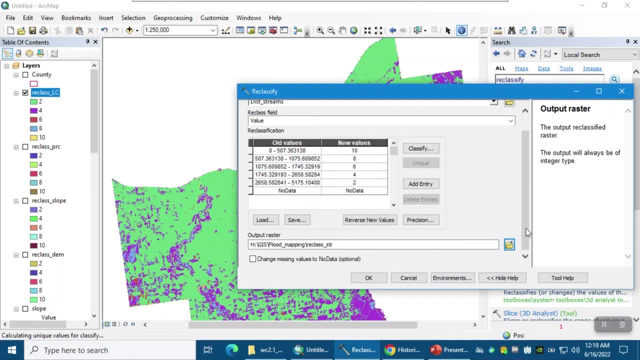 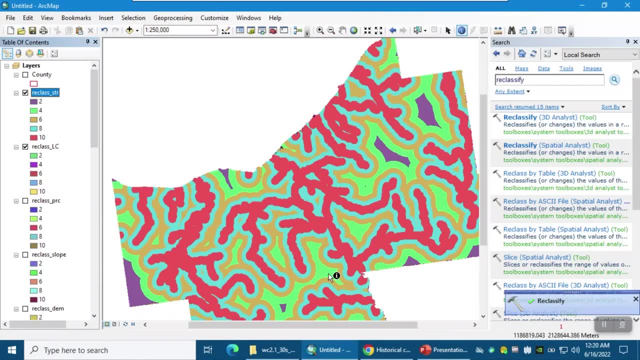 stream or str. okay, and change missing values to no data and then click OK, All right. so now we have reclassified all layers, which means all layers are unitless and they have been rated or scored. So the next step is that we have to combine. 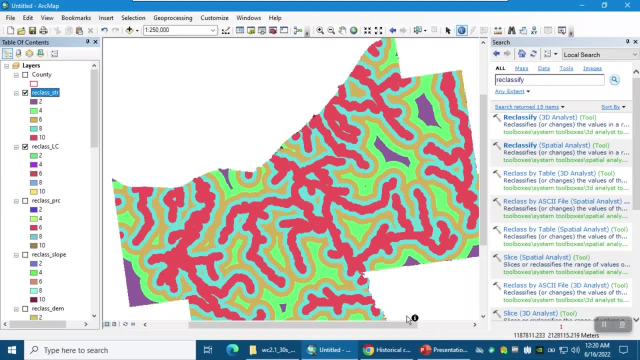 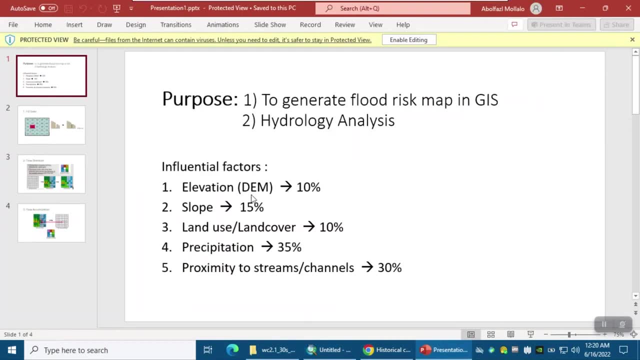 these reclassified layers based on the rates, based on the given rates, based on the opinion of the experts that here we mentioned. Elevation has 10% slope, 15%, 10% for land cover. Precipitation is the most important one. 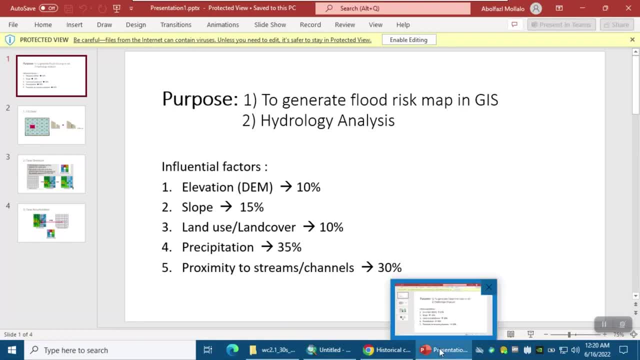 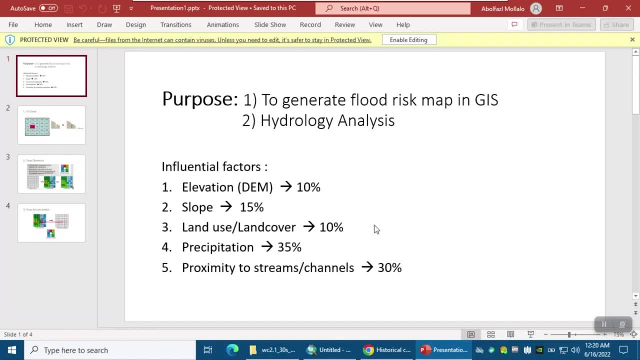 so this is based on the reclassified, and then we have to combine all the factors. After you prepare all of the factors reclassified- which means that you rate them, you make them unitless- the next step is that we have to combine them. 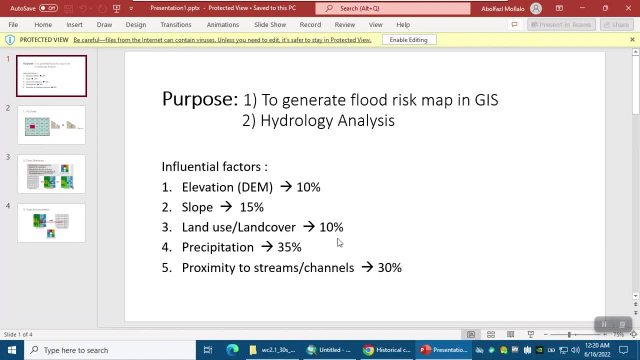 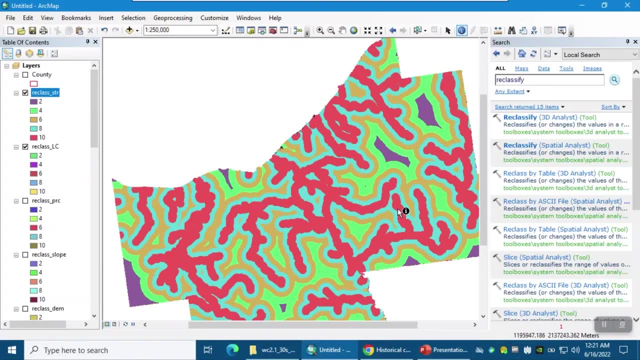 based on the given rates, according to the opinion of the experts. So again, you can use a raster calculator that we did that for the last time. or another way, or more user-friendly way is to use a weighted sum function. so if you type weighted sum, 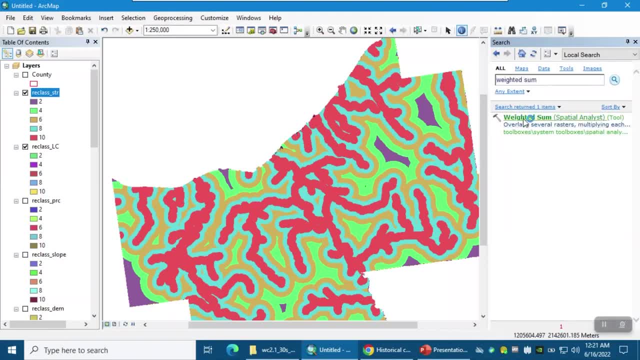 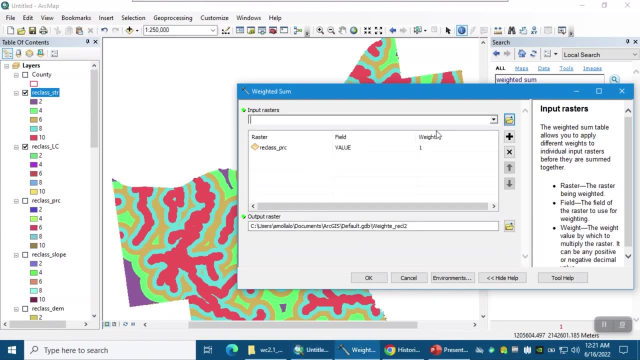 so if you type weighted sum and here you can directly give each raster the weights, okay. so for example, we had reclass for precipitation, we had reclass for streams or distance to streams. we had reclass for streams or distance to streams. 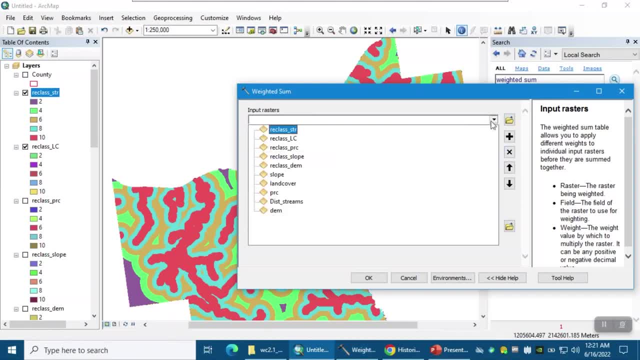 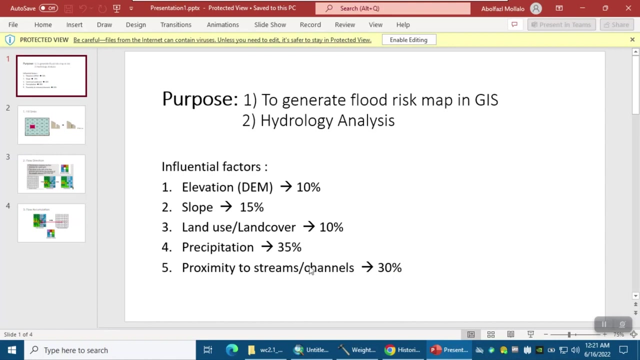 then we had- so let me remove this one- reclass for slope and reclass for digital elevation model and finally reclass for land cover right. So for the precipitation was 35%, so let me see the total has to be 100,. 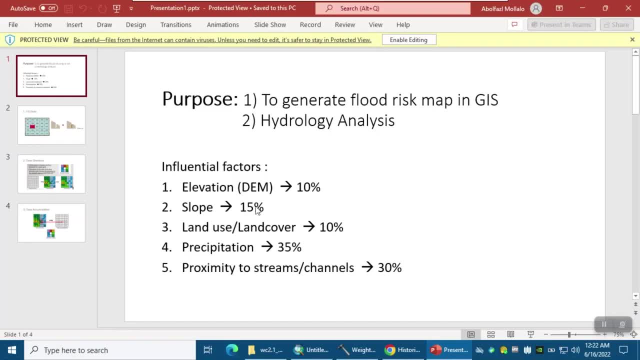 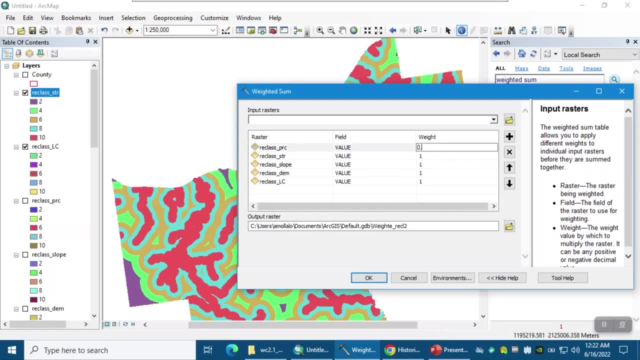 35,, 30,, 65,, 75,, 85,, 90, and 100.. So here is gonna be 35%, 0.35, and reclass for distance to streams is 30% and reclass slope is 15%. 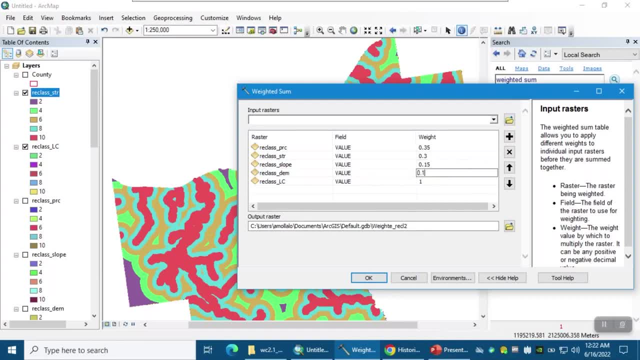 and the last two are 10%, right? If you add them up, the total is gonna be 35,, 65,, 75, plus eight. five is 80, and 90, and 100%, And so this is going to be your final flood risk, right. 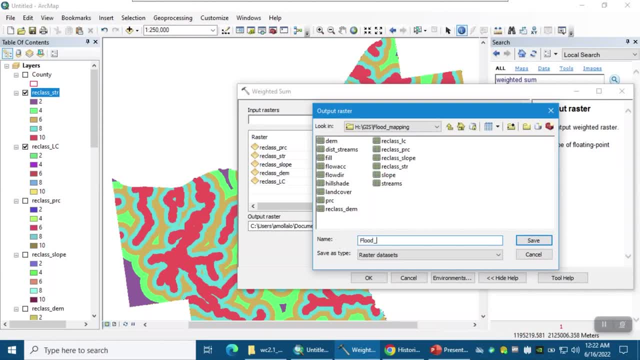 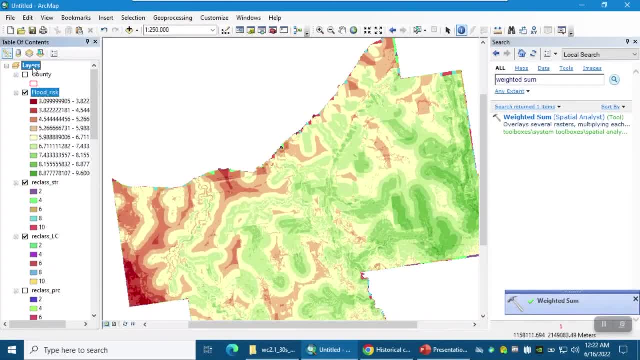 Flood underscore risk and then click OK. So this is: let me uncheck all layer, turn all layer off and flood risk. So here we can see that in the western- sorry, the eastern- part of the study area you have higher chance of flood. 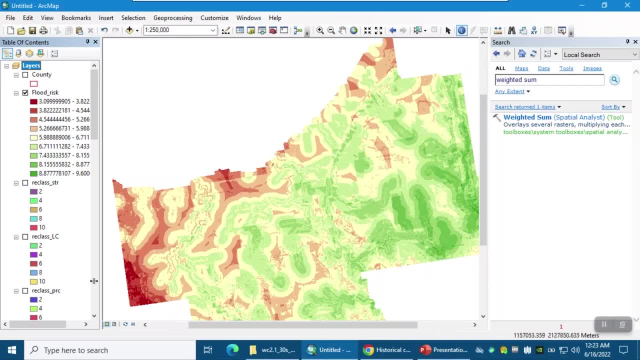 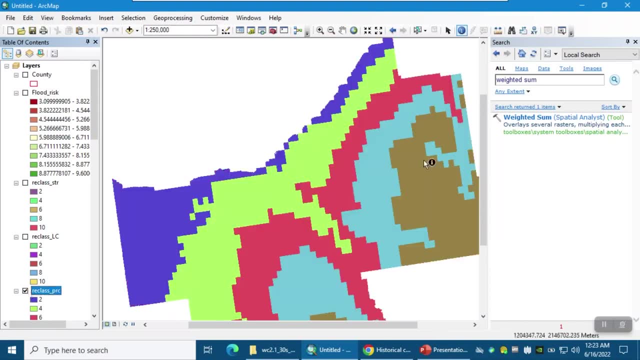 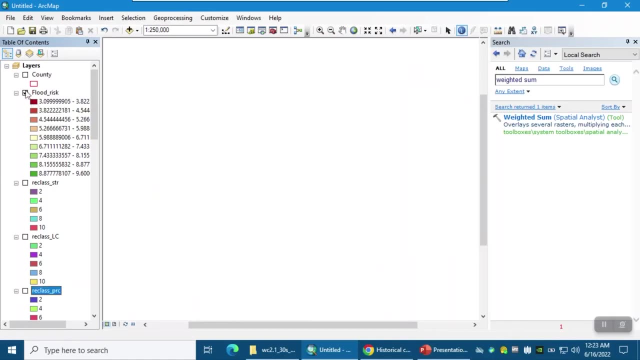 because also here we had the higher precipitation, if you remember. So here we have the chance of precipitation because precipitation was the most important factor. that's why we are in these areas, compared to the western part that had the lower precipitation. 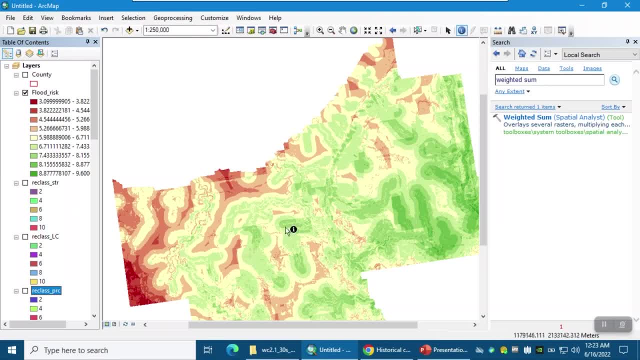 So it kind of makes sense, because the precipitation was the most important factor, And so that's how we can create a risk map for the flood. However, in the future, it would be okay to consider some other factors, like soil type, like vegetation cover. 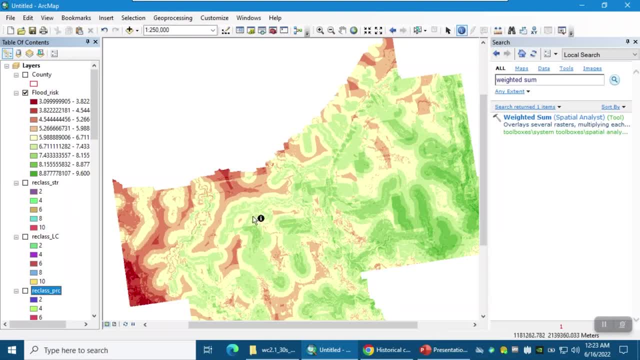 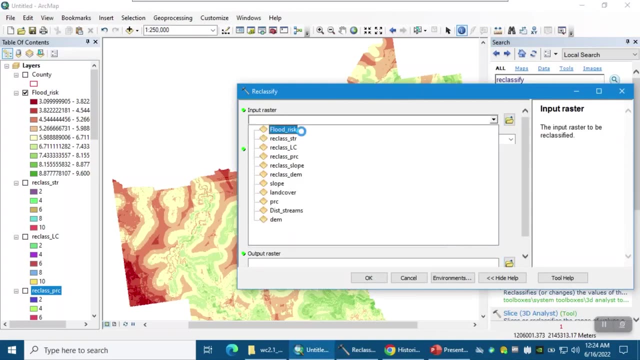 like, for example, normal difference vegetation, like precipitation index NDVI, that we will obtain that from satellite images in the future maps, So we can also reclassify this flood risk map. So let me reclassify it. So I'm gonna reclassify this flood risk. 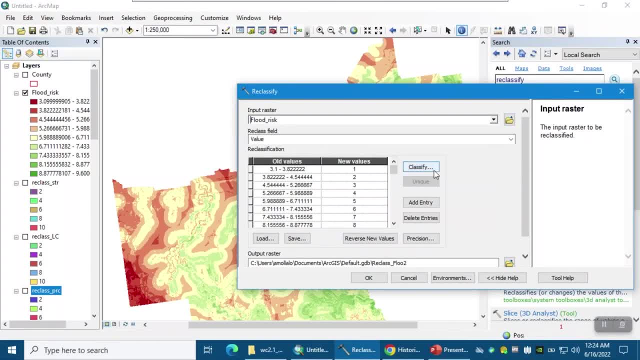 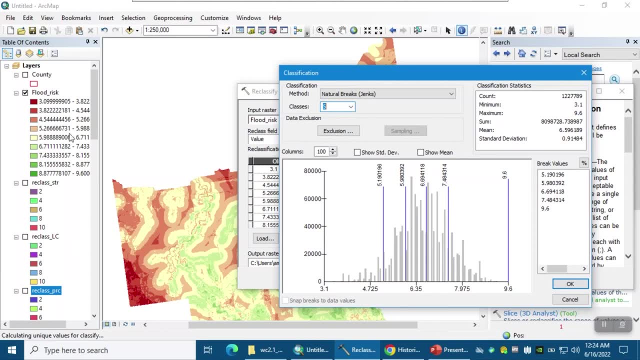 into five classes based on the natural break. So the values are. so, as you can see, the values are starts from three to 10.. So which is like three to 10.. So which is like three to 10.. 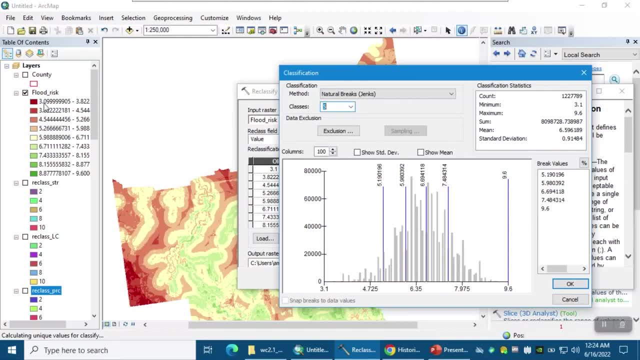 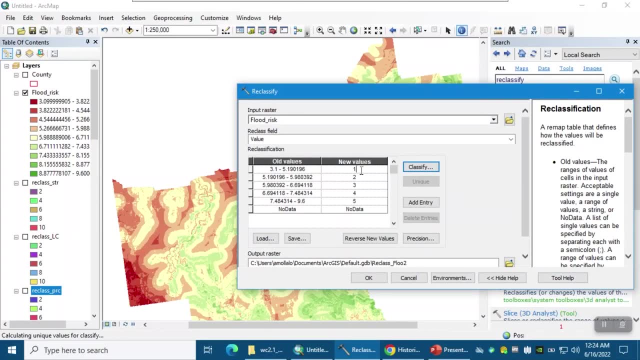 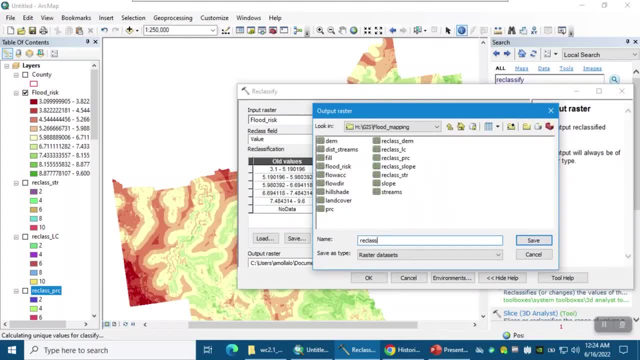 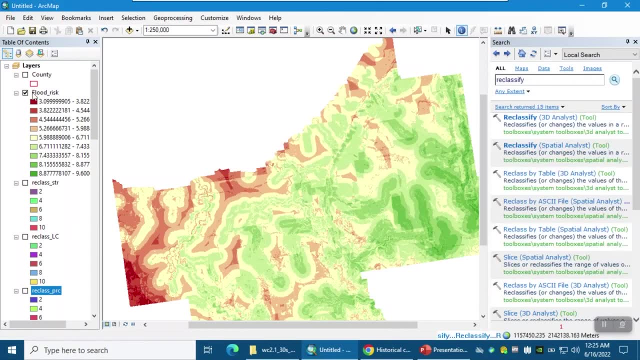 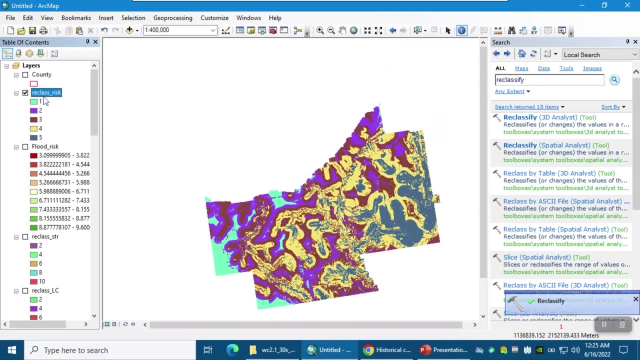 or 30%. here is 96% compared to the other areas, So click OK. So here the value one is low, okay, and then okay. so here is going to be your- uh, the chance of flood. okay, so let me change the symbology. 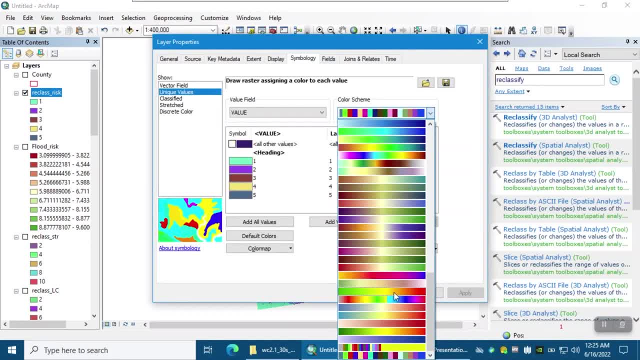 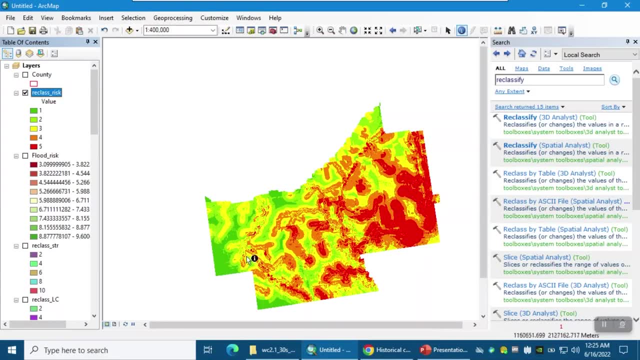 use a better color, okay, so in these areas we have higher chance of flood compared to the these areas, because here we gave higher weight, because here we had higher precipitation- and precipitation was the most important factor, according to the opinion of the experts- compared to the other. so, depending on the 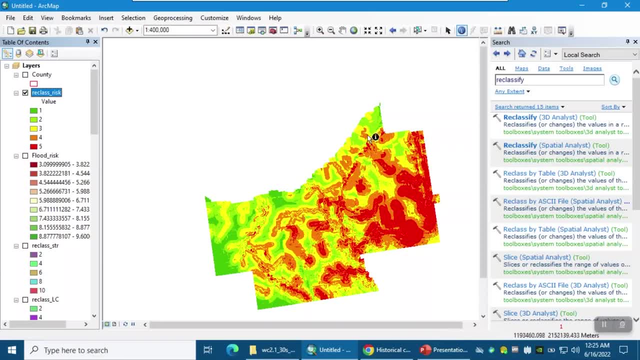 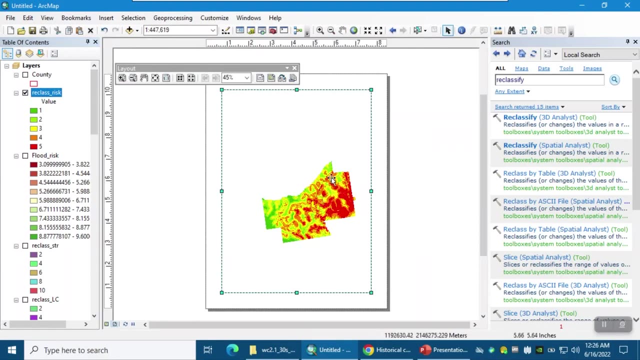 weights that you give to the layer, you will have different layer, a different risk map and also depends on the months of the precipitation. final thing is that you can create. so if you go to the layout view, so here we can create the risk map, you can add. so, for example, you can add the title: